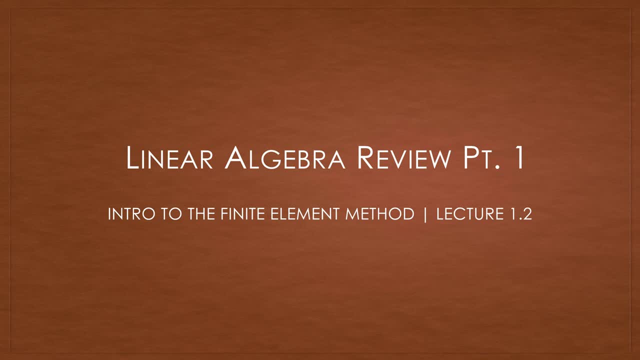 But don't worry, we're going to keep it very simple, very straightforward, with the focus of the finite element method. As you guys may remember, linear algebra- they love to get into those infinite dimensions, stuff like that. Well, we're not going to really do that here. We're going to keep it applicable to our highest dimension, which, of course, is the third dimension, Because if you're designing a building for the fourth dimension, well, something's probably very, very wrong. So the purpose of this linear algebra review isn't to teach you guys linear algebra. 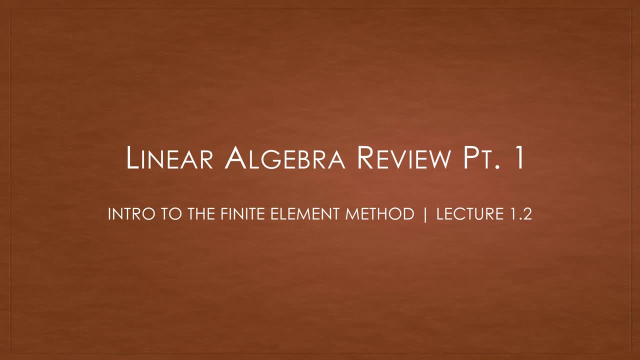 You guys should know the basics by now, be familiar with it. love it or hate it, You guys should know it. What this is meant for is when we get into the solid mechanics review, we're going to be going over a lot of proofs, And a lot of those proofs utilize linear algebra. So it's just to become familiar with the proofs or the operations. So when we get to the proofs, you guys will have a good idea of where the stuff comes from, what exactly I am doing to obtain these proofs. All right, let's get started. 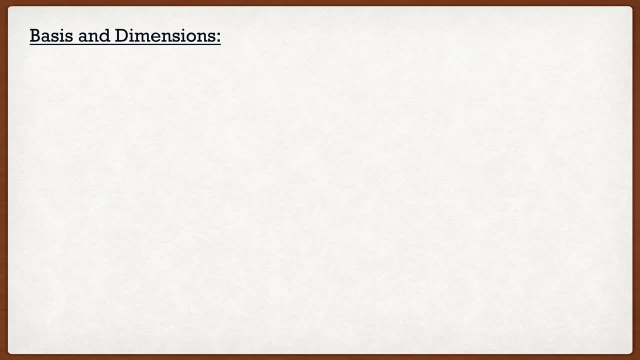 So the first thing we're going to talk about is basis and dimensions. So when we talk about a basis and a dimension, we have infinite dimensions, But of course, we're going to keep it applicable. We're going to talk about two dimensions. The first one is R2, which is a two-dimensional vector space. Now, what exactly does this mean? Well, it means that everything can be written as a linear combination of the vector 1: 0 and the vector 0: 1.. And you guys saying Clayton? well, that doesn't really make too much sense. Let's look at an example Again. over on the right side, we have our vectors. We have E1 and E2, which are the vectors 1, 0 and E2.. 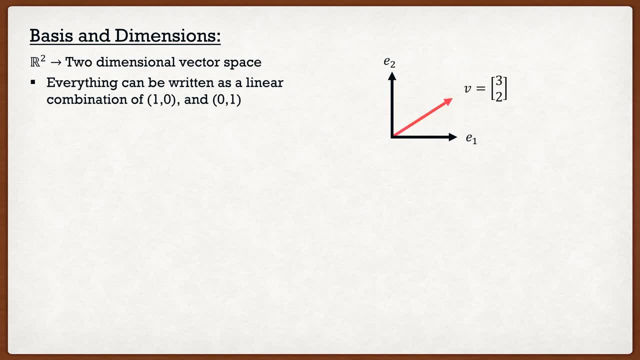 and the vector 0, 1.. And if we have a vector in here which we denote as v or you can name it whatever you want, really, let's say we have a vector v which is 3, 2.. Well, we can take this. 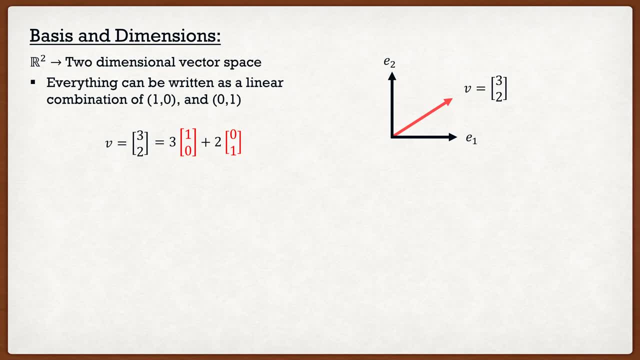 vector and actually express it as a linear combination of those two basis vectors. So we have 3 times the basis vector 1, 0, plus 2 multiplied by the basis vector 0, 1.. So this is important because those basis vectors which I call e1 and e2, they are called basis vectors. 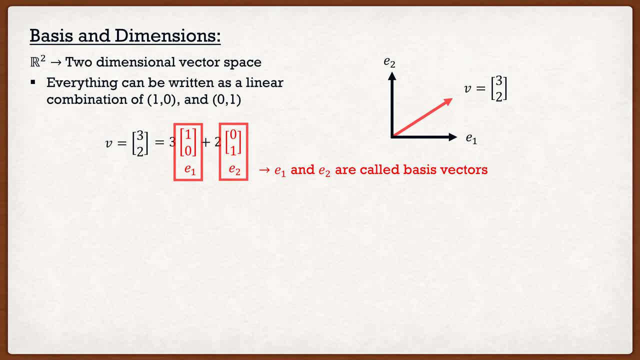 because, again, we can write every vector in that space as a linear combination of those two vectors. Now we have a third dimension, which we call R3, which is a three-dimensional vector space And, just like before, the reason why we call it R3 is because everything can be written. 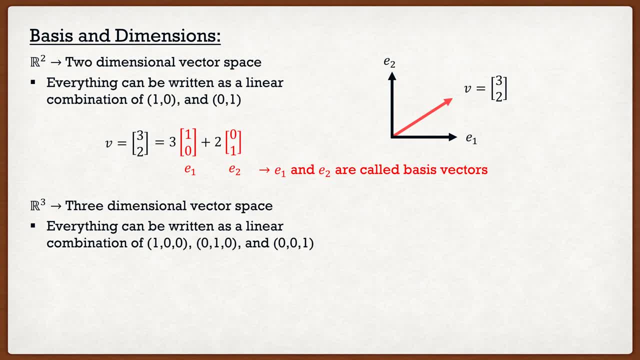 as a linear combination of three vectors. So in this case it could be 1, 0, 0, 0, 1, 0, and 0, 0, 1.. So if we were to look at an example, we have a vector v in the three-dimensional vector space. 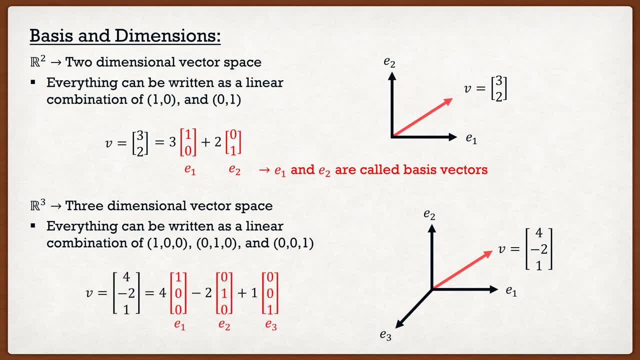 which is 4, negative 2, and 1.. Well, I can actually decompose this vector into a linear combination of the three basis vectors. So this is basis and dimensions, something that's probably fairly obvious to you guys, but it's going to be very important as we discuss later on. Now let's get into perhaps the most. 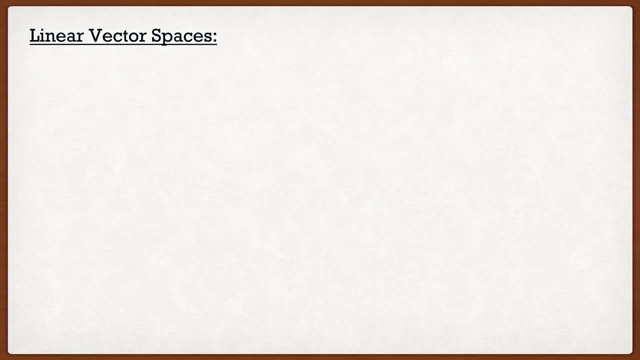 abstract thing, which is linear vector spaces. This is where students really start to hate linear algebra. I know personally. this is where I'm like: okay, okay, I'm not going to be able to understand anything in this course, But I find, with some illustrative examples, 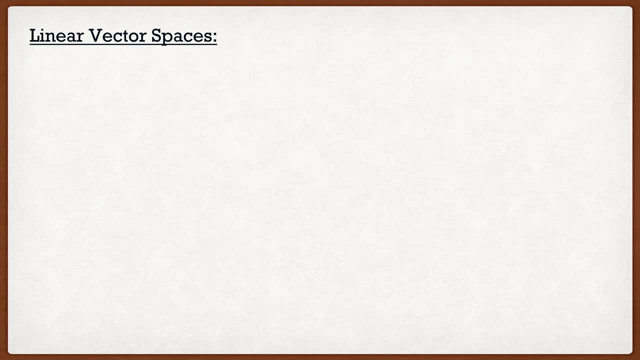 it can be pretty easy to see what a linear vector space is. So a linear vector space is a set of vectors- v- and two operations, such that the following axioms hold for every u, v and w that are vectors, and alpha and beta, which are simple scalars. The first one is, if I were to take two 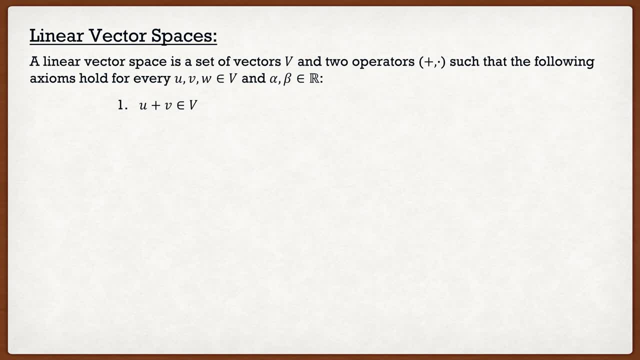 vectors u and v and add them together, well, the resultant vector must also be a part of that vector space. Now, this one is one of the most important ones, But just looking at it, it's not. it looks a little bit confusing. So we're going to discuss more on this in the next slide. 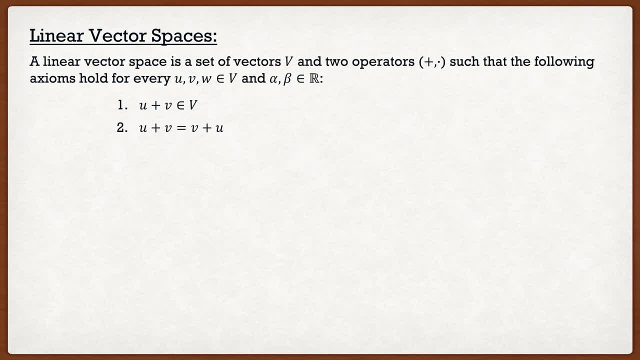 The second one is u plus v must be equal to v plus u. The third one is u plus and then in brackets v plus w must be equal to the brackets of u plus v plus w. The fourth one is there is a zero vector in the vector space And if we add that zero vector to any vector in the vector space, it's. 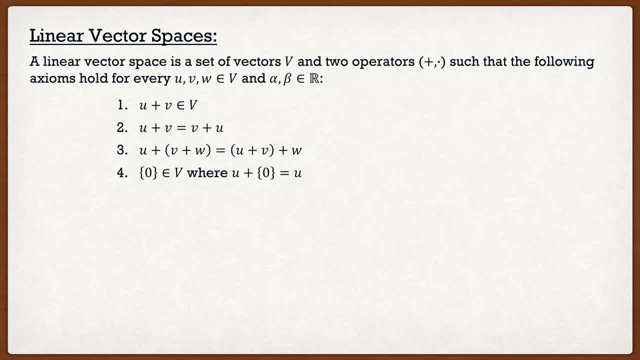 just going to return us with that vector. So if we have u and we add it to the zero vector, well, we're just going to get. u Seems pretty trivial, right, All right. and the fifth one is u plus negative. u is going to be. 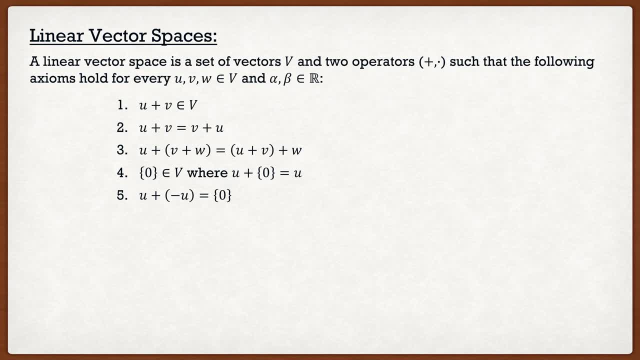 equal to the zero vector. So again, it looks trivial, but these are the axioms. Now, if we look at the first five axioms, they basically have to do with addition. If we look at these, it's always one vector added to another vector. However, it doesn't quite stop there when we're 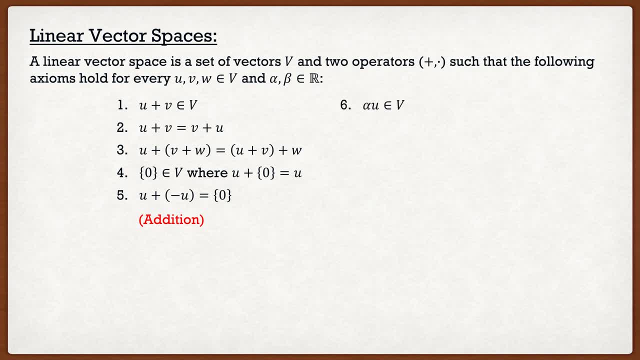 talking about the axioms, We have a sixth axiom which says: if we have a vector in our vector space, u, and we multiply it by a scalar, we're not multiplying it by a vector, we're multiplying it by a scalar. We're multiplying it by a scalar. That resultant vector must also be in our vector space. So just, 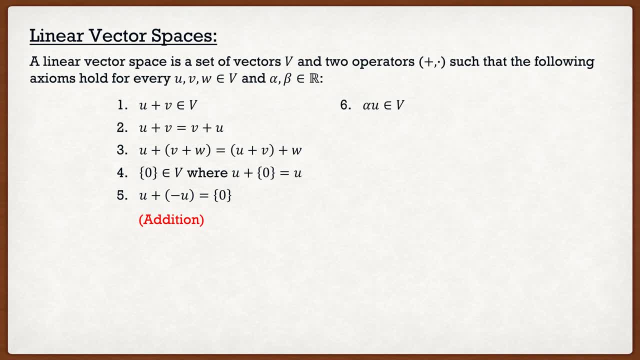 like axiom one on the left-hand side. this is going to be one of the more important ones, as we will see If we move on. if we take a scalar alpha and multiply it to the addition of u plus v, well that can actually be decomposed into alpha u plus alpha v. Moving forward, we can add two scalars. 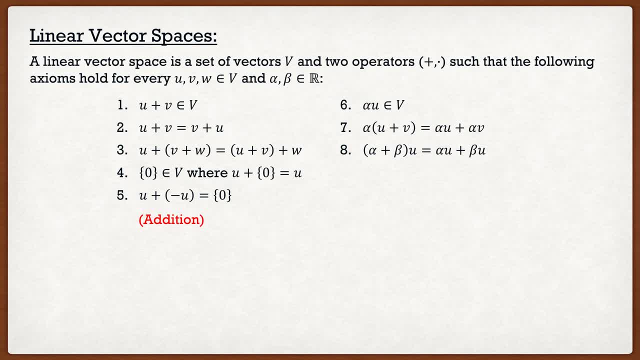 together and multiply by a vector, and that is the same as taking the scalar multiplied by the vector and then adding that to the addition of u plus v. So if we take a scalar alpha and multiply it to the second scalar multiplied by the vector number nine, we have alpha multiplied by beta. u is equal. 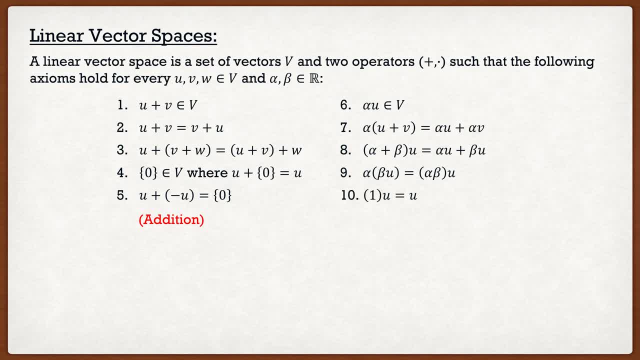 to alpha beta multiplied by u. And finally, if we have a vector u and multiply it by one, well, we're just going to get the vector u. So again, that's one of the ones that seems more trivial. If we look at these next five axioms, so axioms six through ten, we can see that these ones are: 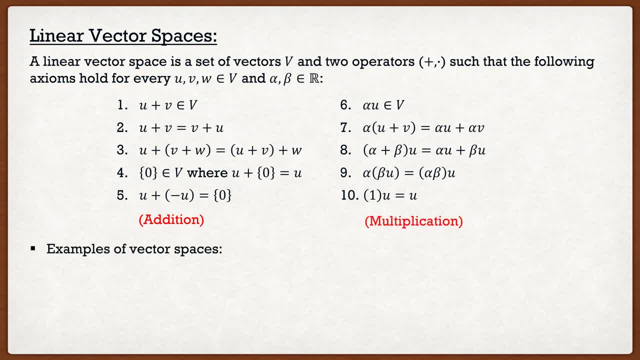 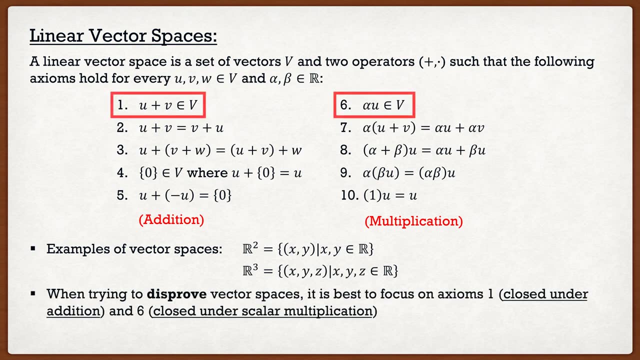 mainly associated with multiplication. Now, some examples of vector spaces include r2, which is a vector xy, where x and y can be anything, or r3, where we have a vector xyz, where xyz, again, can be any scalar. Now, when we're trying to disprove these vector spaces, 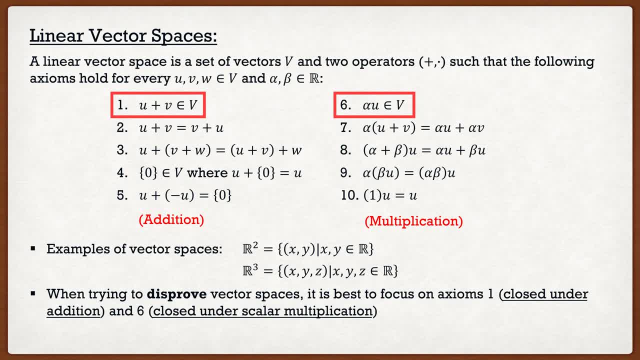 as you guys remember from linear algebra, they love to give you a vector space and say: is this a vector space or is it not a vector space? And if we're trying to disprove a vector space, it's best to focus on axiom one and axiom six, which are closed under addition and closed. 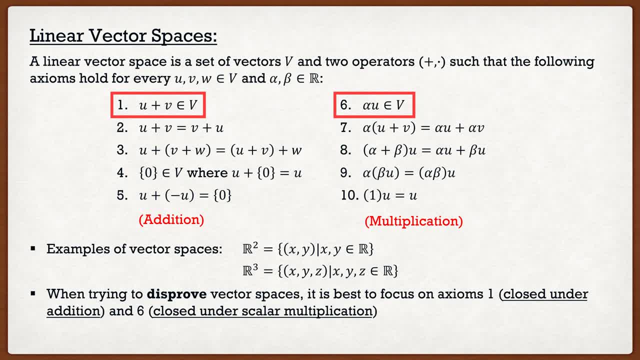 under scalar. So if we're trying to disprove these vector spaces, we can use a vector space to scalar multiplication. Now again, when I talk about this, it's probably very confusing. You're thinking: well, I don't know what a vector space is. So let's look at an illustrative example. 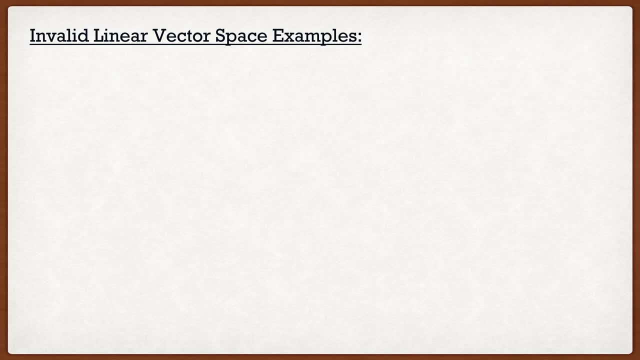 of invalid linear vector spaces. So when they give you a vector space they usually impose some restrictions. Remember in the previous slide when I showed you an example of good vector spaces, we basically said x and y can be anything. or in three dimensions, we said x. 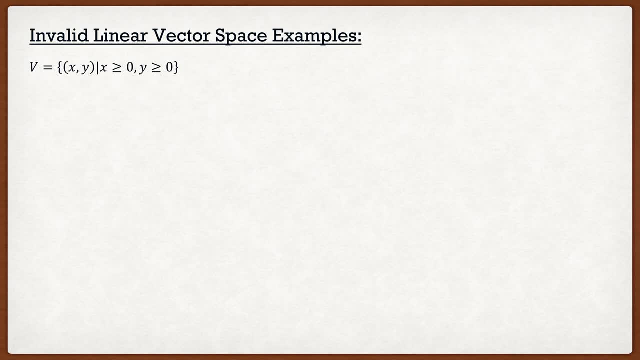 y and z can be anything, So those are always going to be vector spaces. When you start imposing those restrictions, that's when things start to change. So let's say that they give you the vector space x- y, where x has to be greater than zero and y has to be. 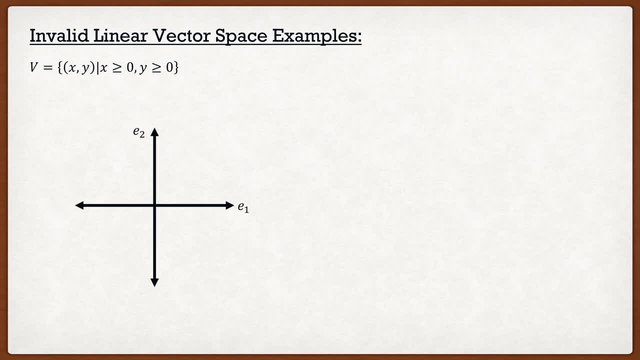 greater than zero. If we were to look at this on a plane and say, all right, if my vector, where both of the components have to be greater than zero, well, I'm basically dealing with this space up here. For instance, if I have the vector two comma one, that's completely valid both of those. 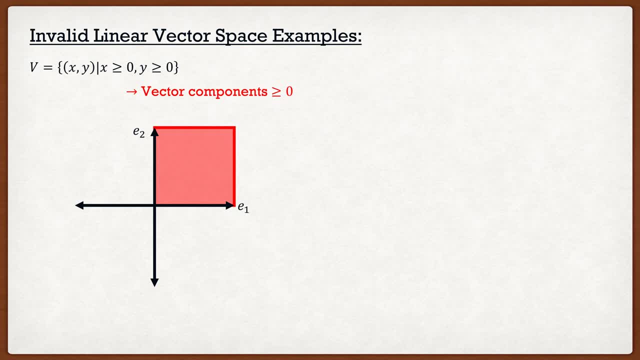 components are positive. However, if I have the vector- let's say negative one comma, negative one- well that vector is actually invalid because those components are less than zero. So when we're looking at this vector space, if both components are negative, we basically have this realm over. 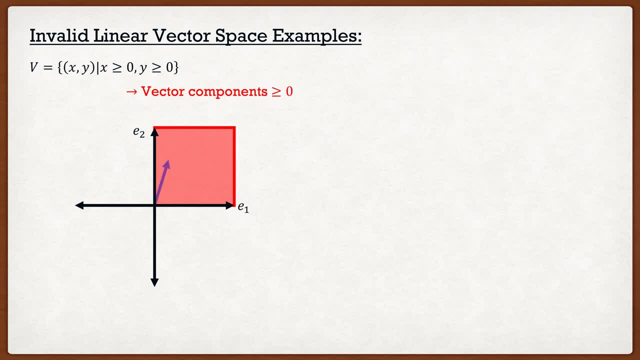 here shaded in red, which is just fine because I can have a vector. let's say I have the vector one comma three. it's in that vector space, it's good to go. If I have a second vector in that vector space, this one, let's say, is three comma one. it's also in the vector space, it's good to. 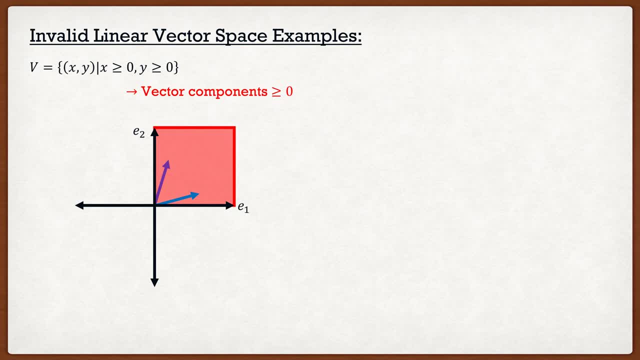 go Now again, when we're trying to disprove vector spaces, we focus on those first two. So the first one is that one that has to do with addition. So if I were to take two vectors in the vector space, in this case we can take a look at the purple vector and the blue vector and we add: 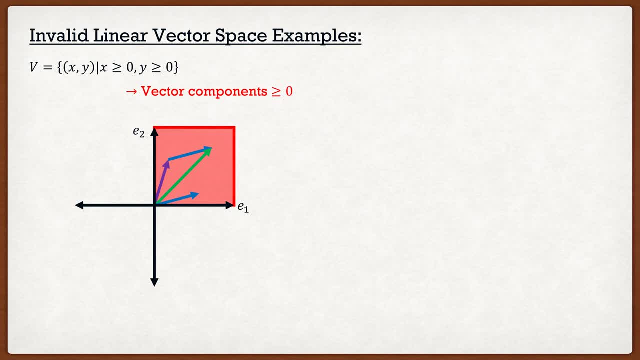 them together, while our resultant vector is going to be that green vector And, as we can see, that green vector also lies in the vector space. So therefore, axiom one actually holds. it's good to go, because any resultant vector we take is also in that vector space. so we're good to go. Now 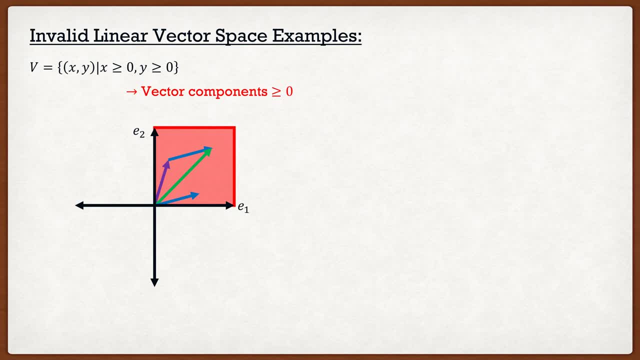 the problem with this vector space is that it's not going to be in the vector space. it's going to actually do with axiom number six, which is multiplication by a scalar. So let's say that we take that purple vector over there and multiply it by two. well, we know that the length of that 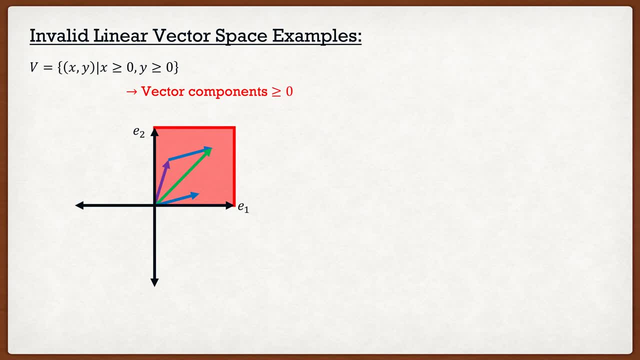 vector is just going to increase by a factor of two, it'll still be in the vector space. However, if we take that purple vector and multiply it by negative one, of course the vector changes directions And, as we can see, the resultant vector in this case is not in the vector space. 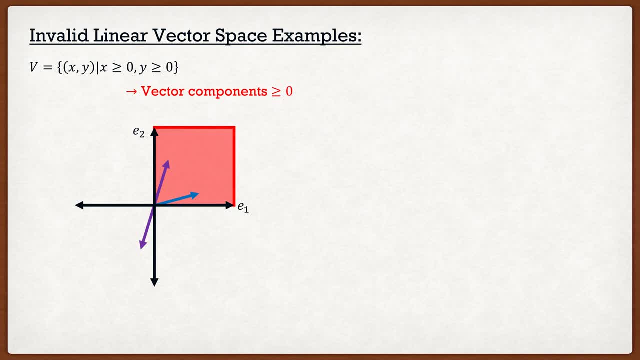 anymore. Therefore this is an invalid linear vector. So we're going to have to go back to the linear vector space because axiom six does not hold in this particular case. So therefore we say this is not a vector space. Now, if we were to look at a different example, let's say that we had the 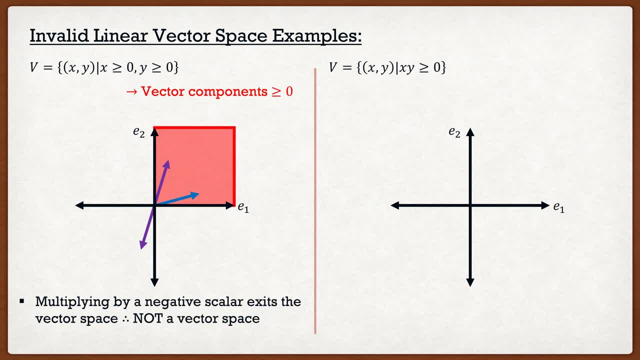 vector space x- y, where the product of the components x times y has to be greater or equal to zero, we can see that we solved the issue we had before, Because if I had the vector two comma two, it's good to go, But if I had the vector negative two, negative two, it's actually still. 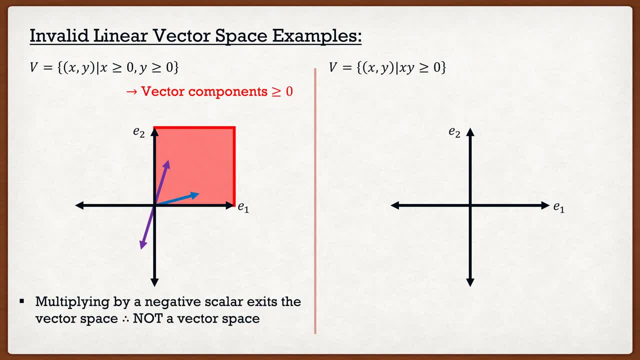 good to go, Because if we take a negative and multiply it by a scalar, we're going to have a negative. we get a positive value. So in this case, the product of the vector components has to be greater or equal to zero, And this means that we actually can work in two quadrants of. 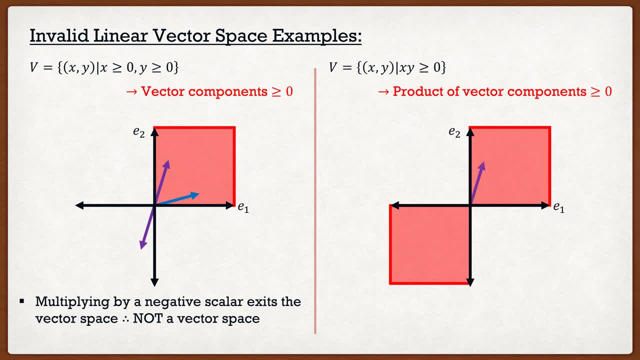 this plane rather than one. So if we have our purple vector there and then we multiply it by negative one, well we get the same result as before, But in this particular case we are actually in a valid linear vector space because of the new restrictions. However, there is a problem. 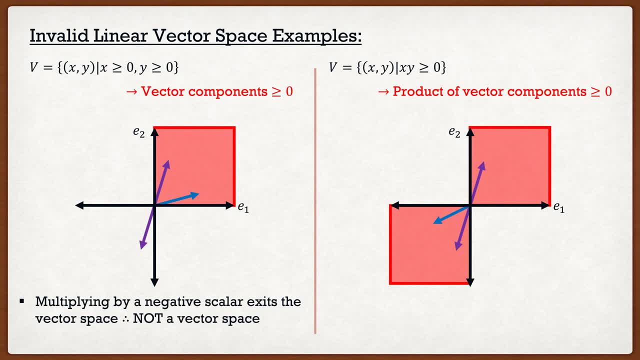 with this linear vector space. So let's take another vector in this vector space. Let's say that this one is negative three comma negative one. So again, it's valid because the product of the components is greater than zero. However, if I were to take this blue vector and add it to the 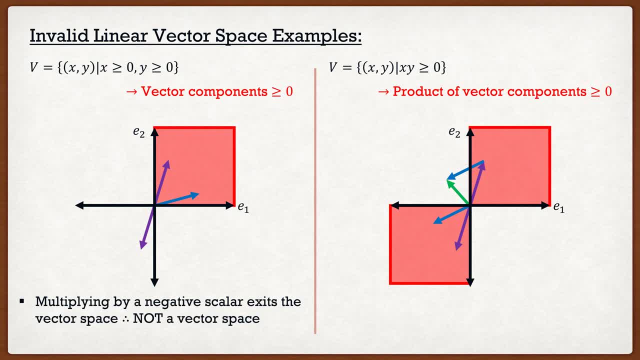 purple vector, as we can see our resultant vector, which is the green vector. that one leaves our vector space. Therefore, adding two vectors can exit the space And we can say that this is not a linear vector space. because of that little fact. 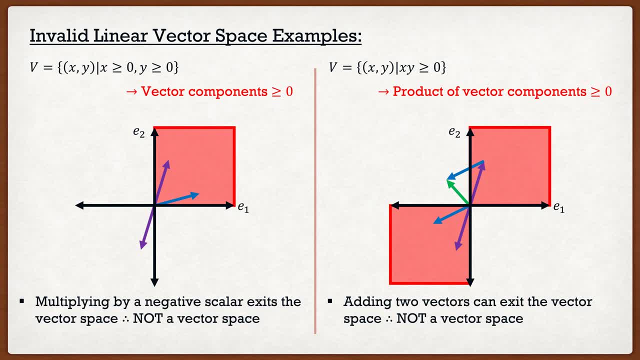 So just a little recap here: If we don't impose any restrictions, chances are you're going to get a vector space pretty easy. It's when we start imposing these restrictions when we start exiting the vector space and result in invalid linear vector spaces. Now I want to keep this transparent. 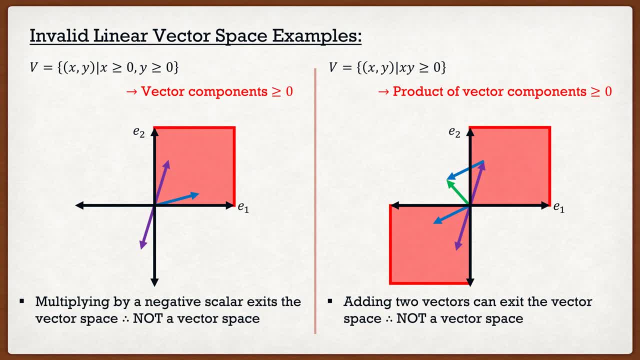 to you guys. Again, we're dealing with practical things in engineering. We deal with R2 and R3. We don't really have these restrictions So technically we'll always be in a linear vector space. We don't have to worry about trying to prove linear vector space. We don't have to worry. 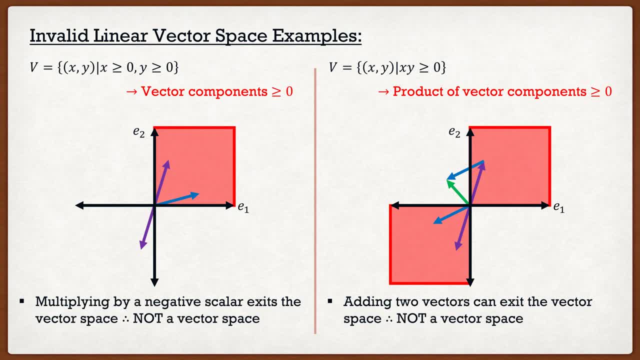 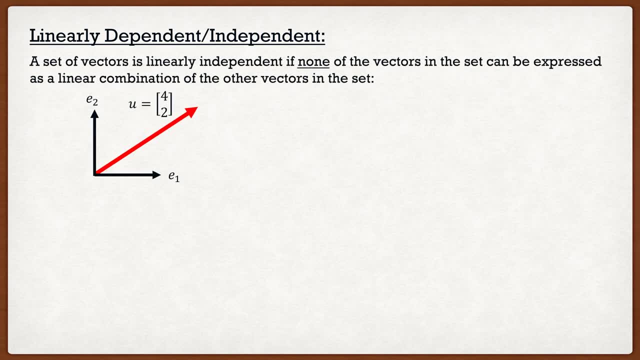 about trying to prove linear vector spaces in this course. That's a little bit outside of the scope, of course. All right, so the next thing we're going to talk about is linearly dependent, slash independent. So a set of vectors is linearly independent if none of the vectors in the set 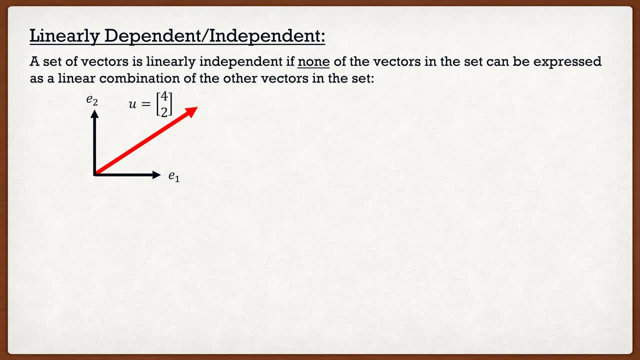 can be expressed as a linear combination of the other vectors in the set. Well, Clayton, what exactly does this mean? Let's take an example. Let's say that we had the vector u, which has the components 4, 2.. Now let's say that we have a second vector, w, which has components 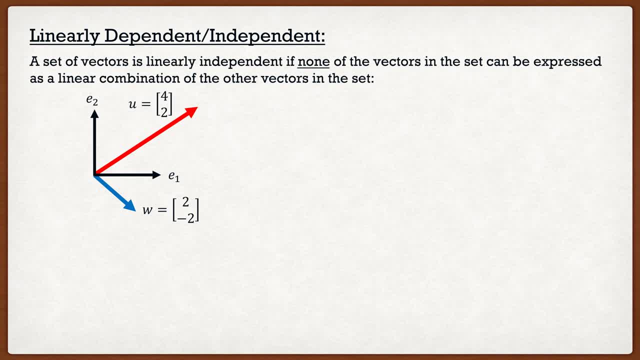 2, negative 1.. Now, just by looking at this, we can see that the directions of these vectors is completely different. Therefore, we would say that these vectors are actually linearly independent, because one vector cannot be expressed as another vector or a linear combination. 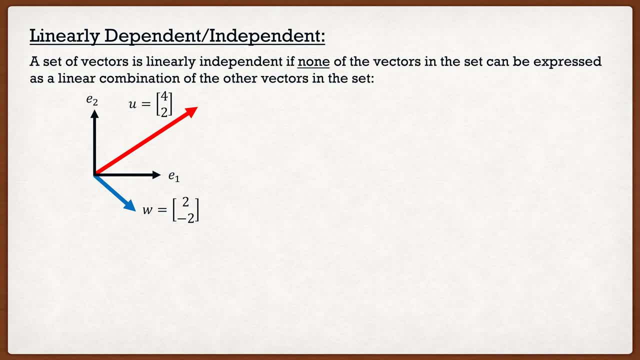 Now you guys may be saying: what exactly does it mean to be expressed as a linear combination? Let's look at a third, vector v, which shares the exact same direction as vector u. These vectors would actually be linearly dependent because if I were to take the vector u, which is the vector u, 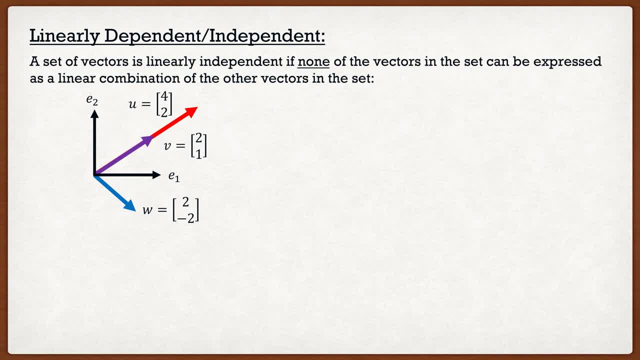 and I'm going to take the vector u, which is the vector u, and I'm going to take the vector u, which is the vector v, which is 2, 1, and multiply it by the scalar 2,. well then, I end up with the. 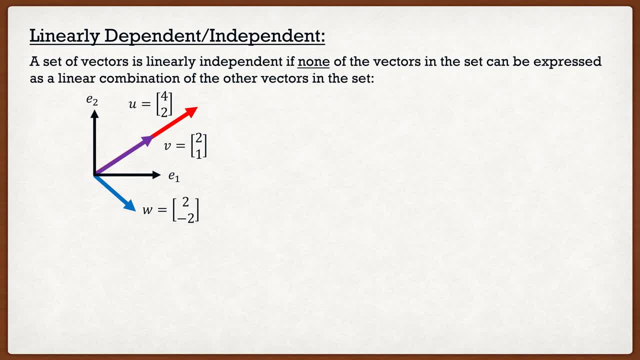 vector 4, 2, which is the same as vector u. Therefore, if we want to determine if two vectors are linearly dependent or independent, we simply have to solve the following equation: alpha 1 multiplied by vector u plus alpha 2 multiplied by vector v is equal to the zero. 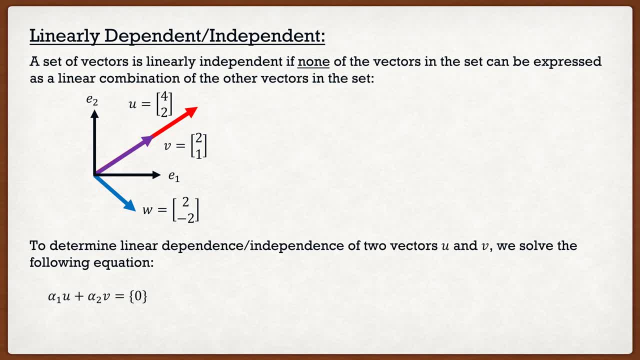 vector. So the goal here is: we're going to solve for alpha 1 and alpha 2, because of course we know the vector u and we know the vector v and of course we know the zero vector. If you guys don't know the zero vector, well, 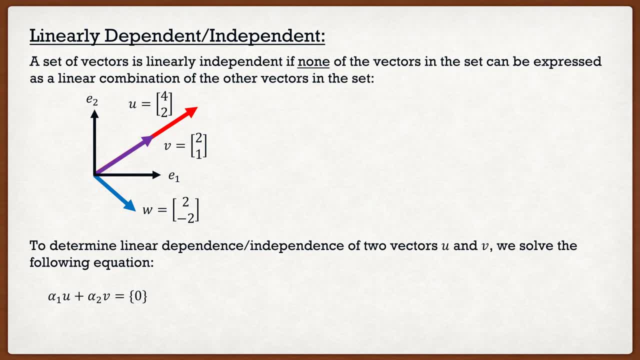 then we have bigger problems. So there's going to be two solutions or two cases when we solve this problem. One is: alpha 1 is equal to alpha 2,, which is equal to zero. Therefore, the vectors are linearly independent: Alpha 1 equal to alpha 2, which is equal to zero. This is, of course. 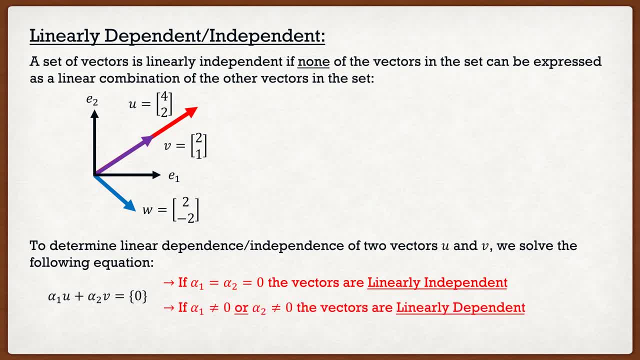 the trivial solution. so this makes sense. The second case is: alpha 1 does not equal zero or alpha 2 does not equal zero. Now notice the or here: As long as you have one of these coefficients not equal to zero, we can say that these vectors are linearly. 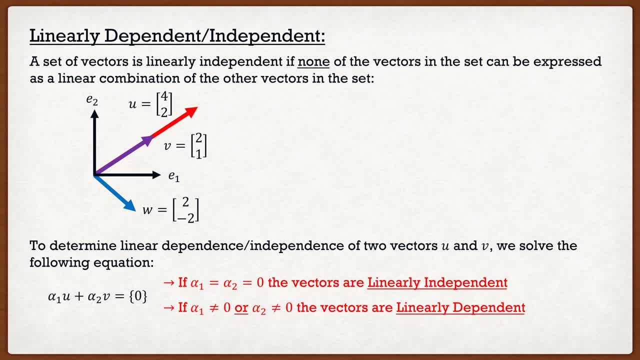 dependent. And if we were to go up to our case above, we can actually see this. Let's take the vector alpha 1, or, sorry, the vector u and the vector v, which we already said are going to be linearly dependent. If we were to solve the equation alpha 1 multiplied by 4, 2. 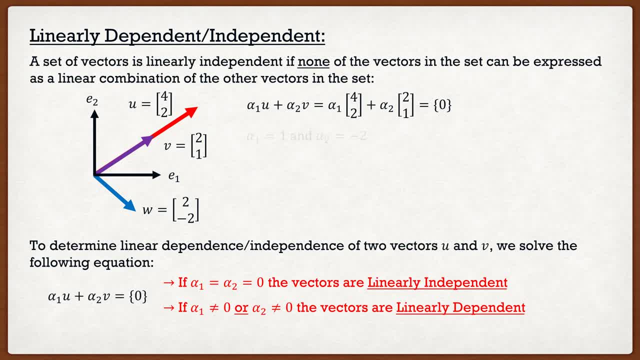 plus alpha 2, multiplied by 2, 1 is equal to the zero vector. I can have a solution where alpha 1 is equal to 1 and alpha 2 is equal to negative 2. And since these are both not equal to zero, we know that u and v are linearly dependent. On the other hand, if I were to look 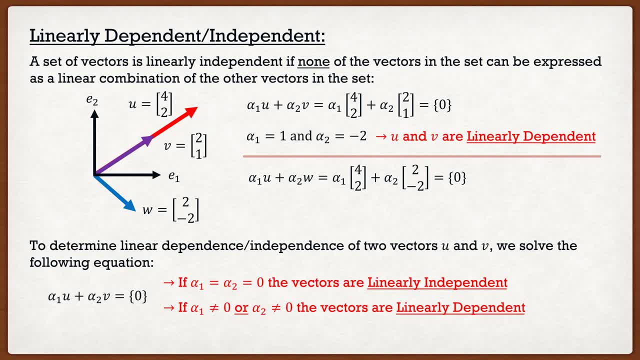 at the vectors u and w, which we already agreed that they are not linearly dependent. so therefore they are linearly independent. we are to look at the equation here. We have alpha 1 multiplied by 4, 2 comma 2, plus alpha 2 multiplied by 2 comma negative. 2 is equal to the zero vector. Now 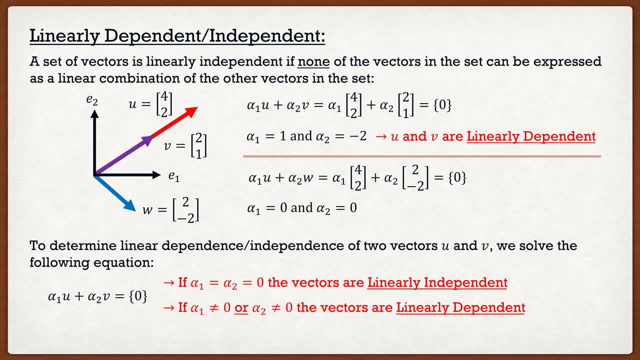 the only way the solution holds is if alpha 1 is equal to zero and alpha 2 is equal to zero, or the term is equal to zero. So if we were to look at the vector u and v, we know that u and v are. 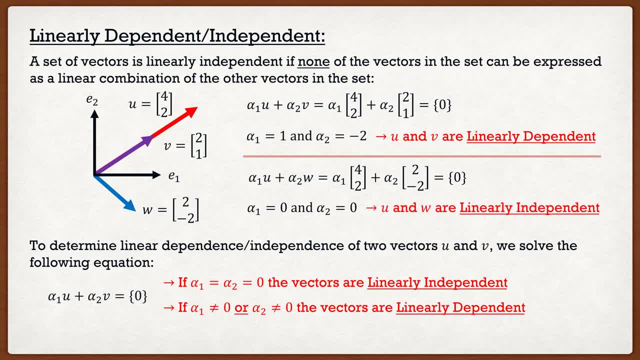 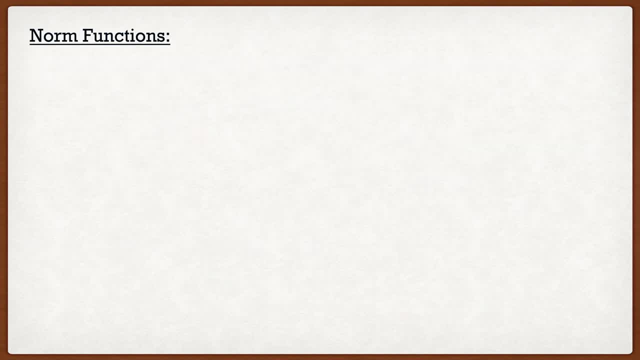 linearly independent. So that's linear dependence slash independence. Let's move on to something a little bit more fun, which is norm functions. So norm functions, as you guys will see in the finite element method, are going to be extremely important. The reason why norm functions are: 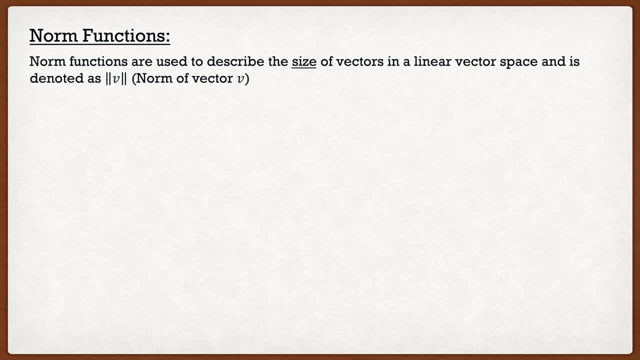 used to describe the size of vectors in linear vector spaces, and it's typically denoted as what I call the double absolute value sign of v. So this would be considered the norm of vector v. Now you guys may not have a vector v, Let's say you have a vector a. It's the same. 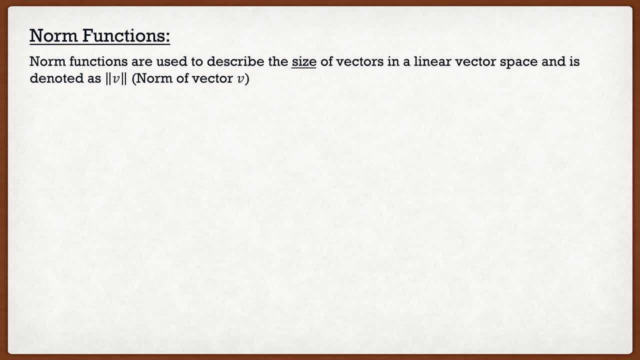 thing. You just put those double absolute value signs around it. It means that it's going to be the norm of that vector. Now a norm function must satisfy the following for any two vectors, u and v, and any real scalar alpha. The first one is positive scalability, which basically means if 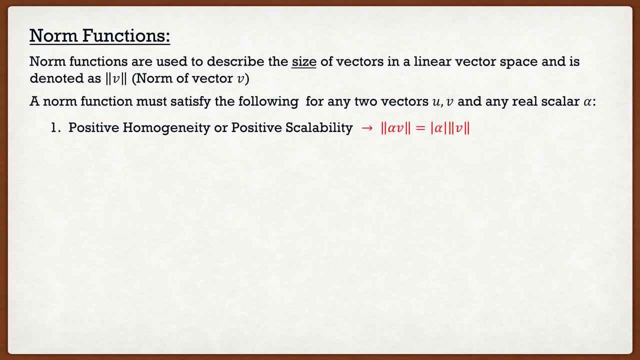 I were to take the norm of alpha v. well, this is the same as taking the absolute value of a and then multiplying it by the norm of alpha v. So if I were to take the norm of alpha v. the second one is the triangular inequality, which says that the norm of vectors u plus v. 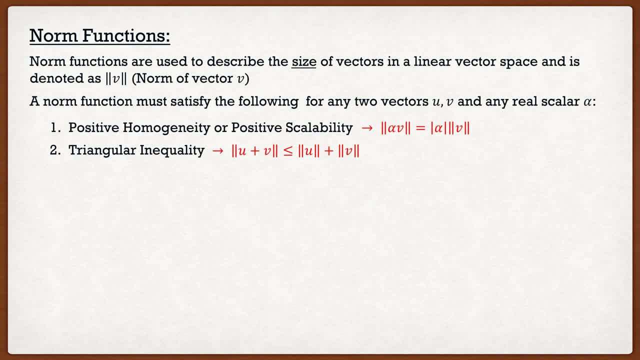 is less than or equal to the norm of vector u plus the norm of vector v. And finally the third one, positive definiteness, which basically says: if the norm of a vector is equal to zero, well then that vector has to be the zero vector. There is no ifs ands or buts with that one. 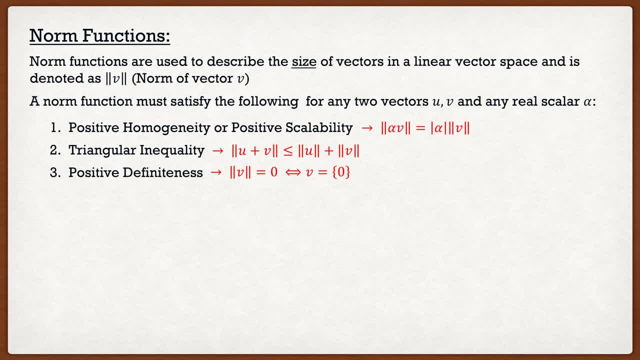 It's just kind of a straight up statement. Now, if we look at these three requirements, actually a lot of different functions that satisfy these, So there isn't one definite norm function. However, in this course, when we deal with the finite element method, 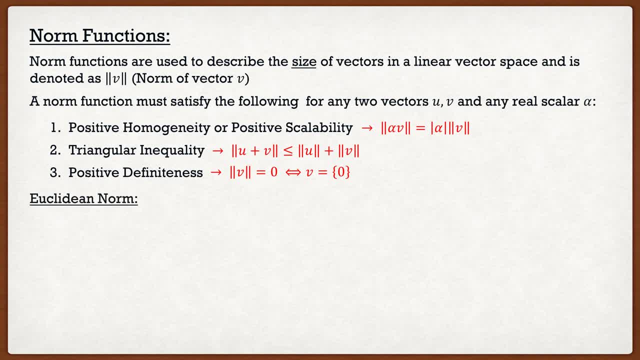 we are going to look at one in particular, which is called the Euclidean norm. Now, it sounds really complicated, It sounds really gross, but this is actually probably the norm function you guys are most familiar with, And that is if we have a vector v with components v1,, v2,. 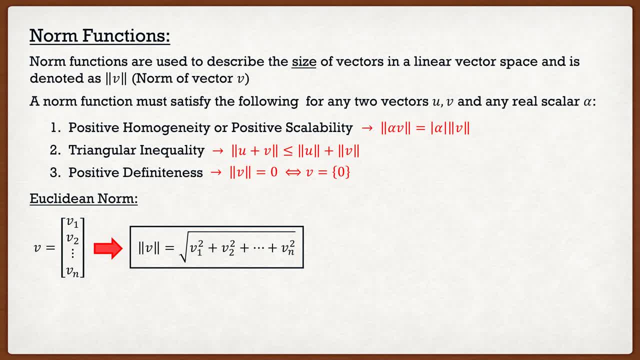 all the way to vn. well, the norm of that vector is simply going to be all the components squared, summed and then square rooted. So this is something you guys may have seen a lot all the way back into your first year of university when you guys were dealing with statics even. 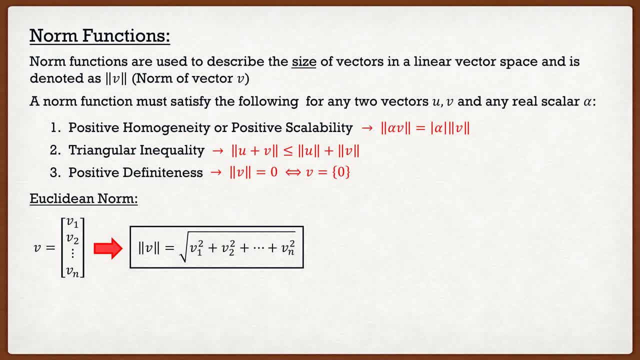 where if we wanted the magnitude or the length of a vector, we would use this formula. So the magnitude, length of a vector. it's the same thing that we're doing here with Euclidean norm. So if you guys hear me say the norm of a vector, I'm basically just saying the length of the vector. 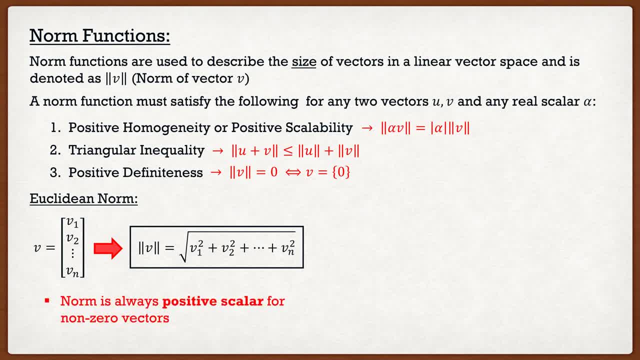 or the magnitude of the vector. Now if we look at the formulation here, we can see that the norm is always going to be a positive scalar for non-zero vectors. So if I were to calculate the norm of a vector and I get, let's say, negative 2, I did something wrong. It's a good indication. 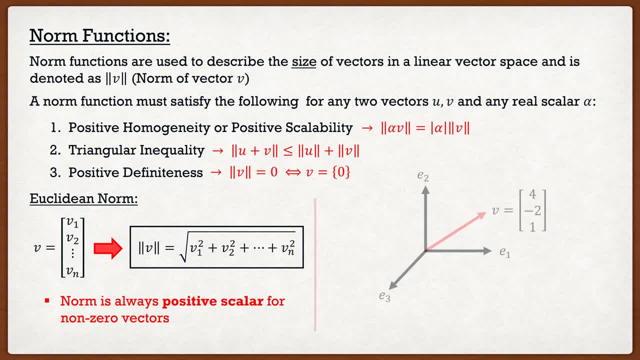 that. hey, maybe I should go back and recheck my answer. Now. let's do a little bit of an example. So let's say that we have this three-dimensional vector v with components 4, negative, 2, and 1.. 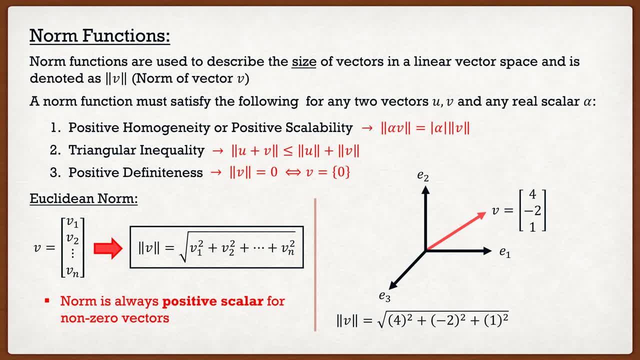 If I wanted the norm of this vector, I would just go 4 squared plus negative, 2 squared plus 1 squared, add up all those components and then square root it I get the norm is equal to around 4.583.. Now what exactly does this mean in the picture? 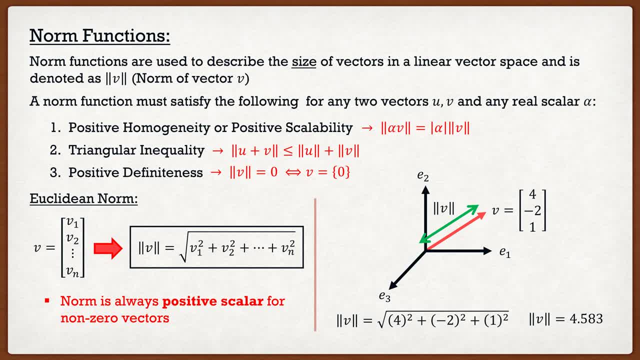 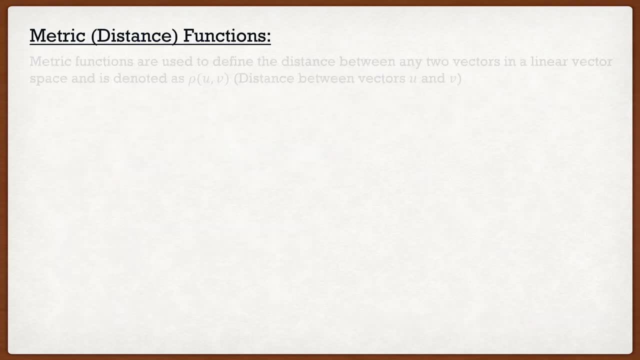 It means that the length of this vector is 4.583 units, So it's very easy, something that you guys should have seen a lot earlier in your guys' career. Again, not too complicated. Now let's go to the second thing, which is a metric or a distance function. So metric functions. 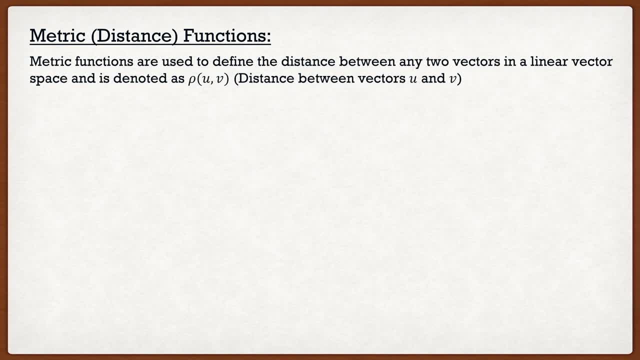 are actually used to define the distance between any two points or any two vectors in a linear vector. Now a metric function must satisfy for any three vectors- u, v and w- One symmetry, which basically means that if I wanted to find the distance between u and v, it doesn't matter if I start at u and go. 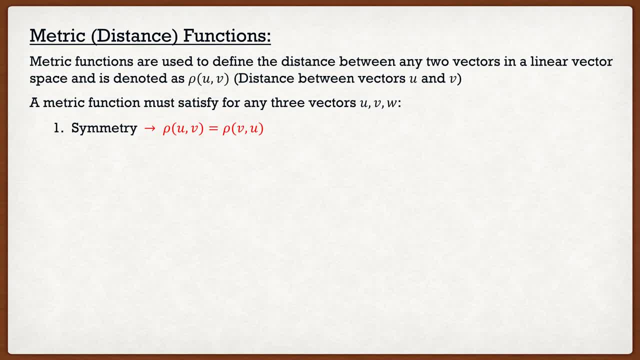 to v, or start at v and go to u. They're going to be the exact same distance. Let's say that I wanted to go from New York to Los Angeles. Well, that's going to be the same distance as going from New York to Los Angeles over to New York. It makes sense. The second one, again, is the triangular. 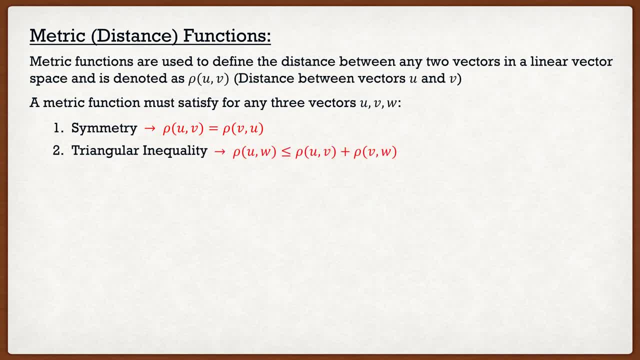 inequality, which means that if I were to go from the distance from u to w, this is going to be less than or equal to the distance from u to v and then v to w. And the third one is saying that if the distance between two vectors, u and v, is equal to zero, then u and v must be the exact same. 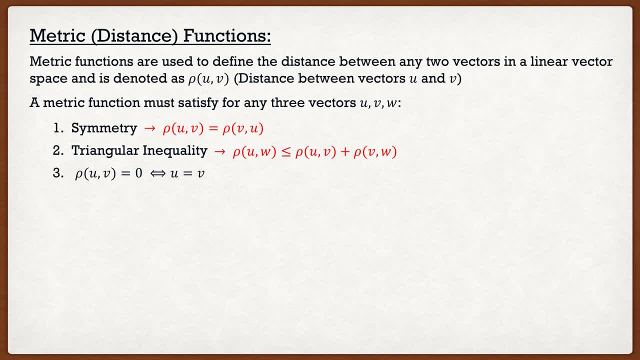 vector Now, just like the norm function. there are many functions that can actually satisfy the three requirements, but we are going to deal with one in particular, which is the Euclidean distance. So this is going to be a common theme. We have a lot of different functions that satisfy. 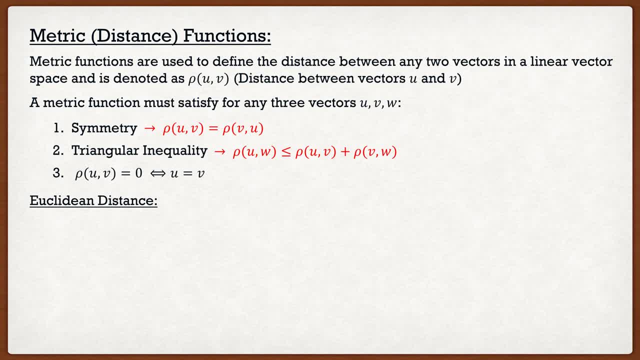 something, but we are always going to look at the Euclidean version of it. Now, the Euclidean distance is nice and easy If I have two vectors, u and v, with components u1, u2, un and v1, v2,. 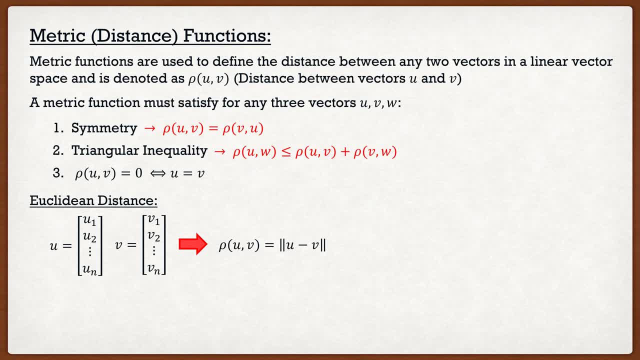 all the way to vn. the distance between them, or rho of u comma v, is simply going to be the norm of u minus v. Now you guys are saying, well, this looks a little bit crazy, a little bit complicated. 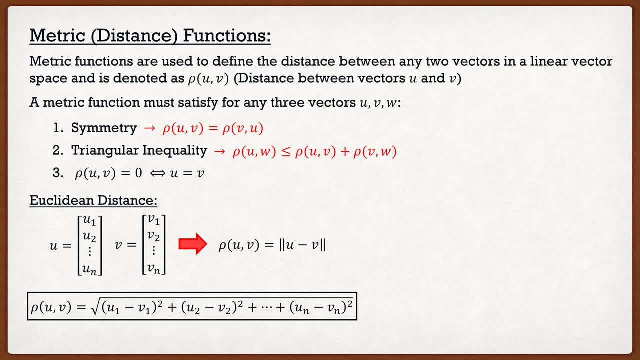 Let's simplify it a little bit. Well, it's simply going to be u1 minus v1 squared plus u2 minus v2 squared plus, et cetera, et cetera, And then we just square root it, So it's actually going to. 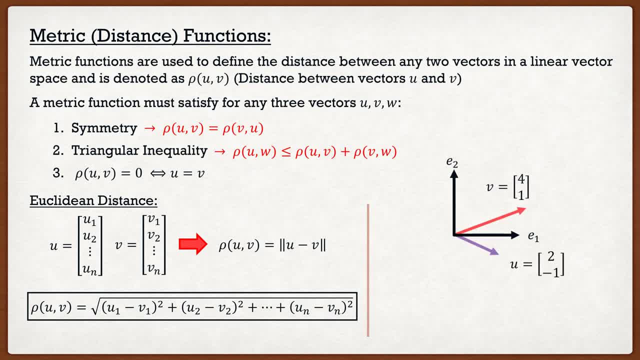 be nice and simple. Now, if we were to look at an example of this, let's say in two dimensions. I had two vectors, u and v, with components 2 comma negative 1 and 4 comma 1.. Well, the distance between them is just going to be 2 minus 4 squared. 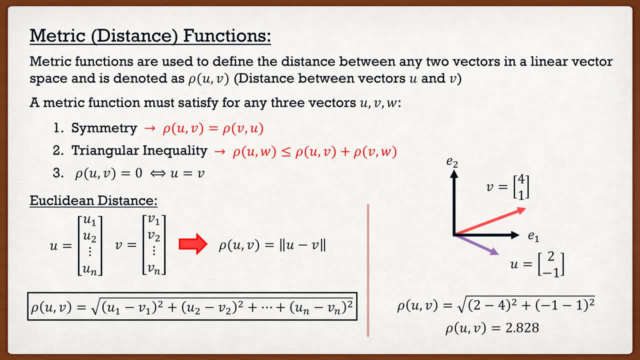 plus v, That's negative, 1 minus 1 squared, and then all square rooted And I get the distance between them as 2.828 units. What does this mean in the picture? Well, it means that the distance between the heads 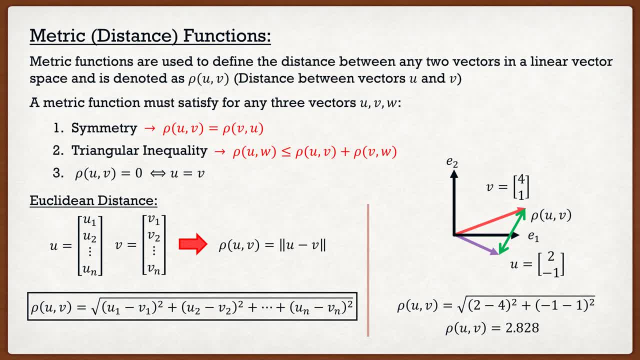 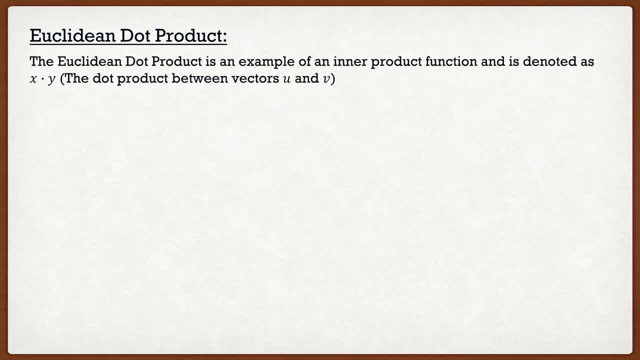 of those two vectors is going to be around 2.82 units, So nice and easy. The last one we're going to talk about real quick is the Euclidean dot product. So the Euclidean dot product is actually an example of an inner product function and is denoted as u dot y. There's a little bit of a. 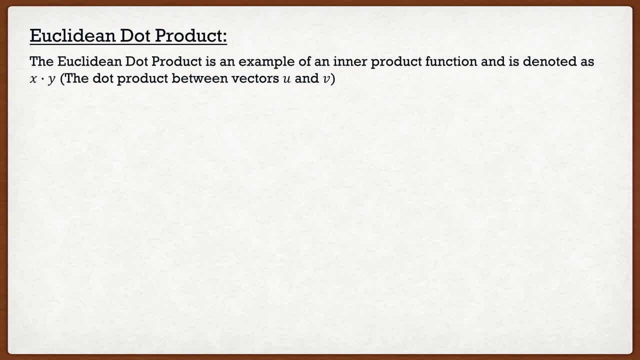 typo here. It says x dot y. I meant u dot y, which basically means the dot product between vectors u and v. Now if we were to look at this, it's actually an example of an inner product function. And what an inner product. 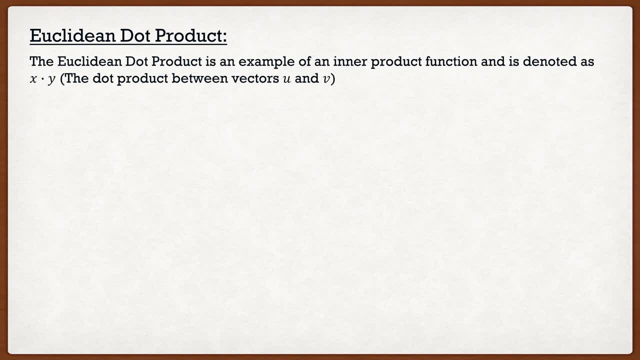 function wants to do is create some sort of geometric relationship between two vectors, And that's what we're going to see a little bit later. But first let's talk about the formulation of the dot product. It's actually really simple, Looks gross. really simple. That's kind of the theme. 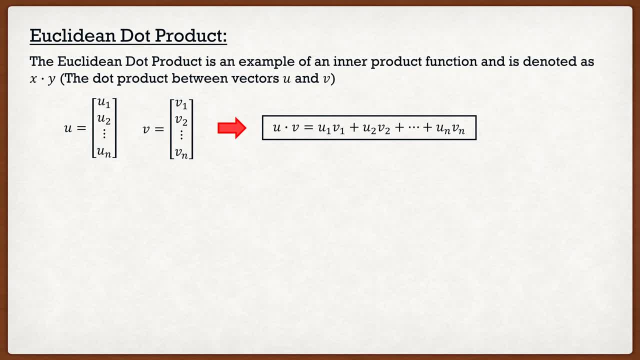 of linear algebra as a whole Looks really gross, actually really simple. Looks gross, really simple. So if I had two vectors, u and v, with components u1, u2, all the way to un, etc. and v1, v2, all the 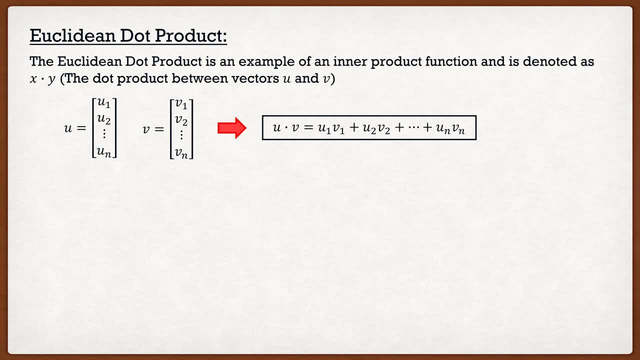 way to vn. well, the dot product between them is actually just going to be each component multiplied together and then summed up. So if I wanted to go u, dot, v, it's going to be u1 multiplied by v1, plus u2 multiplied by v2, plus dot, dot, dot, all the way to un multiplied by vn. The key here: 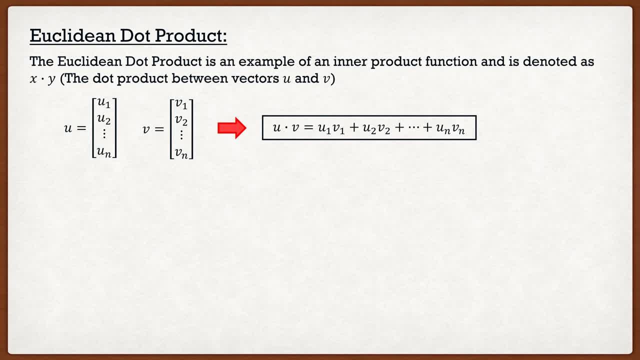 and this is what a lot of students typically forget, mainly in undergrad- I'm sure that you guys are much better than the undergrads- is that we are taking two vectors and we end up with a scalar. So if I were to dot two vectors together and end up, 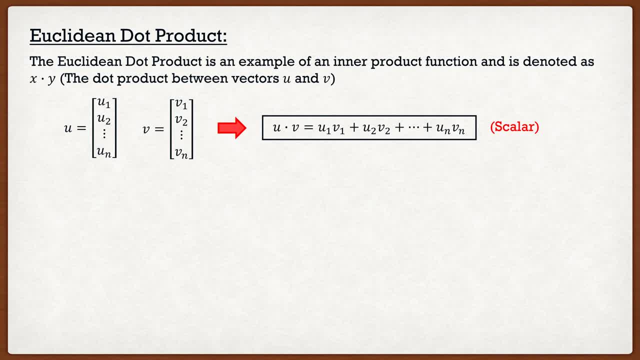 with a vector- again probably an indication. you guys did something wrong. Now, in two and three dimensions, the dot product is actually used to relate the geometric angle between vectors. So again I said that it's an example of an inner product function, which basically means we are: 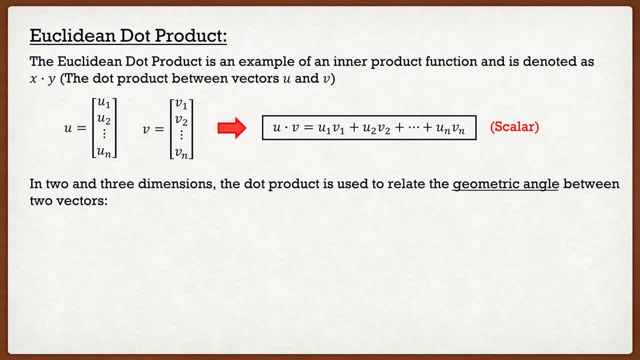 trying to add some geometric relationship between two vectors. So if I were to dot two vectors, so if we were to look at the formulation of the dot product, which is u1, v1 plus u2, v2, etc. well, this is actually equal to the norm of u multiplied by the norm of v multiplied by cosine. 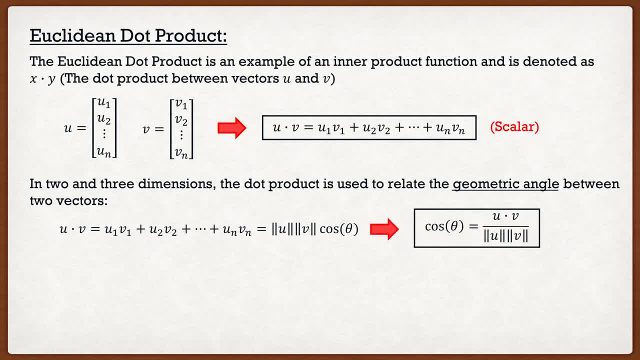 of theta. I can rearrange this formula to say that cosine of theta, where theta is actually the angle between the two vectors, is equal to u dot v divided by the norm of u multiplied by the norm of v. This is great, because if I were to look at a scenario here where I had my two vectors, u and v, 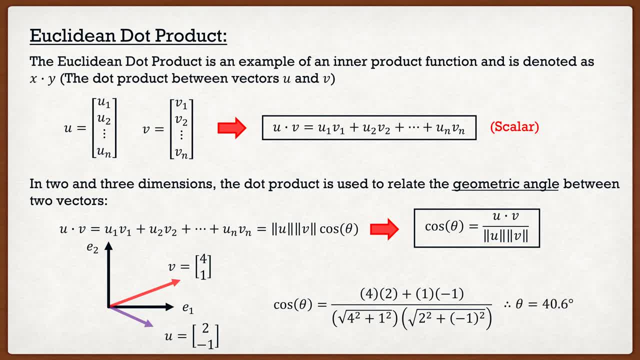 I can actually calculate what cosine theta is and I can find that the angle between these two vectors is actually 40.6 degrees. So if I were to look over at my diagram here, I actually know the angle between those two vectors. Again, really nice, because it takes something complex like a. 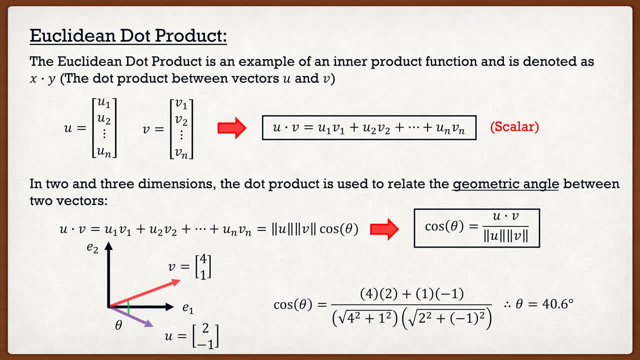 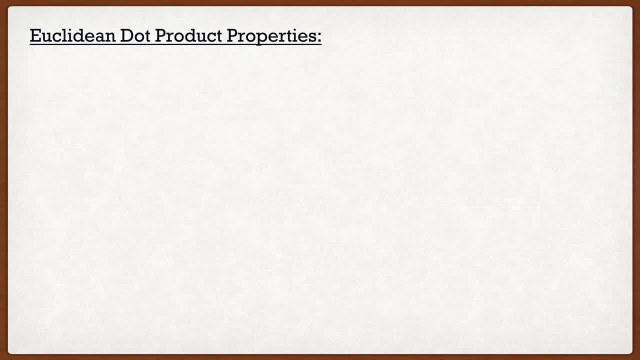 vector and it provides some geometric relationship between them, And geometric relationships are great because they're very easy to visualize. All right, so there are a couple of properties of the dot product that I want to go over. The first one is the angle between the two vectors. 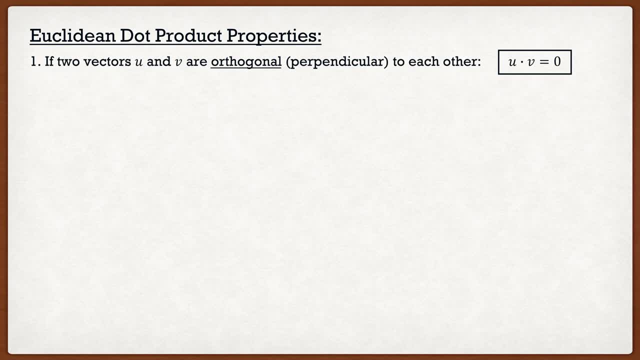 If two vectors, u and v, are orthogonal, which basically means perpendicular to each other, u dot, v or the dot product between vectors u and v is actually going to be zero. This proof is very simple. If I were to look at the formula I had before and look at the cosine of theta, well I say: 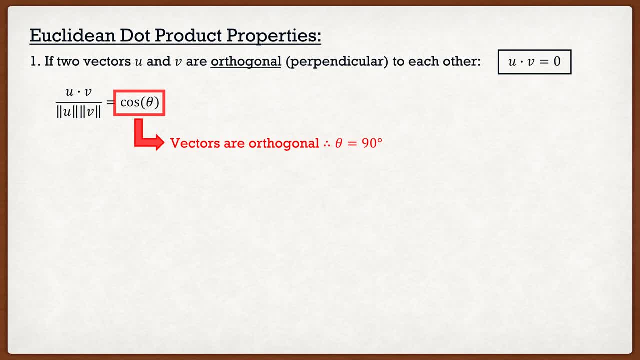 well, the vectors are orthogonal. perpendicular, it means that theta is 90 degrees. Well, if I were to go cosine of 90 degrees, I get zero. Therefore, u dot v divided by the norm of u and the norm of v is equal to zero. I can move the norms to the other side. I get u dot v is equal to zero. So 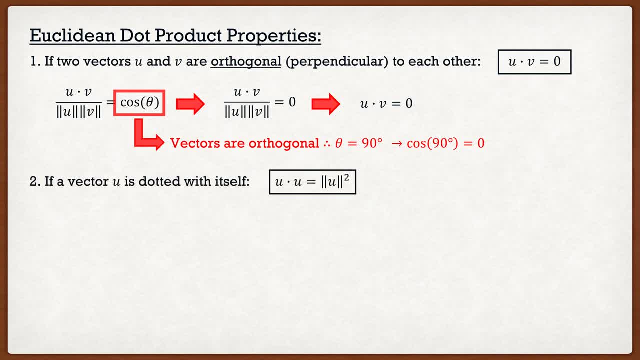 again a very straightforward proof. Now, the second property is if a vector, u, is dotted with itself, so u dot u, it's actually equal to the norm of u squared. And again, proof, very simple. I look at the basic formula, I look at the cosine of theta part and I say if I'm dealing with the same vector, 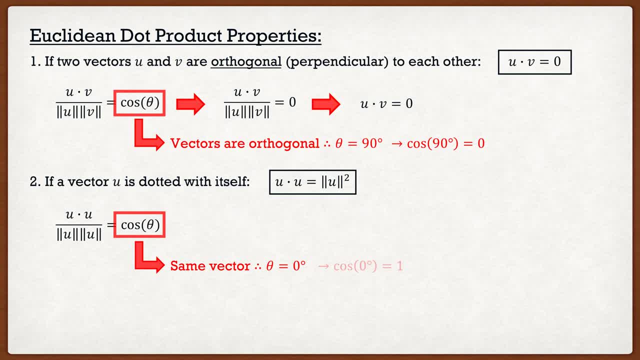 well, there is no angle between them. Therefore, theta is equal to zero. Therefore, cosine of zero is equal to one. From there I can make the formula equal to one. move the norms to the other side where I got u dot. u is equal to the norm of u multiplied by the norm of u, And since the norm 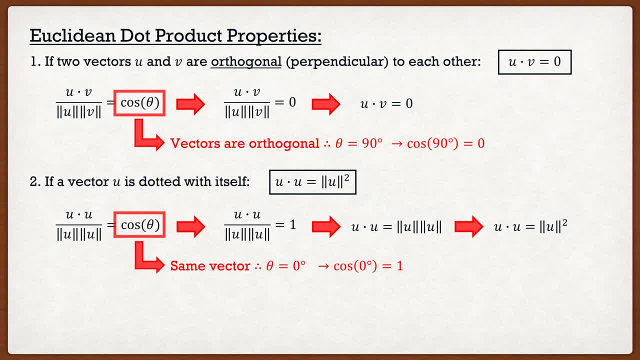 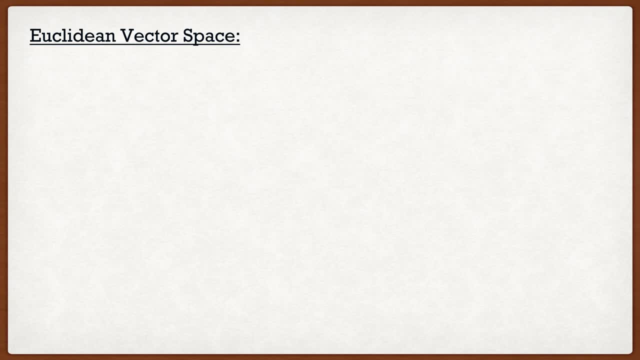 of u is just a scalar, u dot u is actually equal to the norm of u squared. So nice and simple. Now, why am I showing you guys a norm function, a distance function and the dot product? Well, it has to do with Euclidean vector space. So a Euclidean vector space is a vector space equipped. 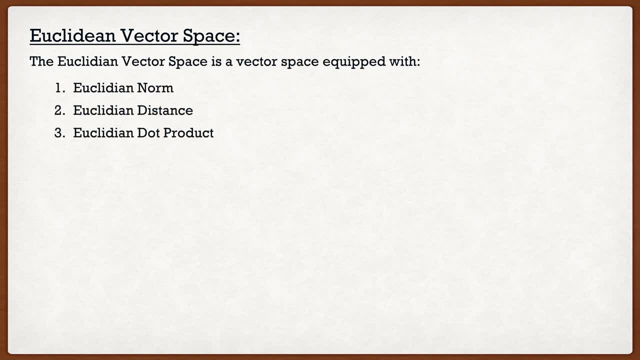 with, as you may have guessed, the Euclidean norm, Euclidean distance and the Euclidean dot product, which we've already discussed. Now, what's special about this is these functions allow for the definition of an orthonormal basis set, which is going to be one of the most important things. 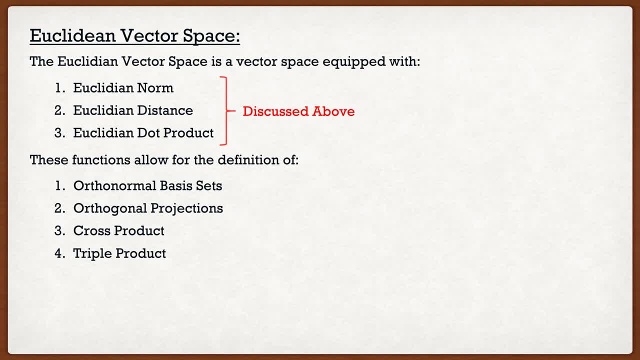 moving forward: Orthonormal projections, cross product and triple product. So the cross product and the triple product will be very important once we start discussing some of the proofs that we see in solid mechanics. But before we get into that, let's discuss what an orthonormal basis 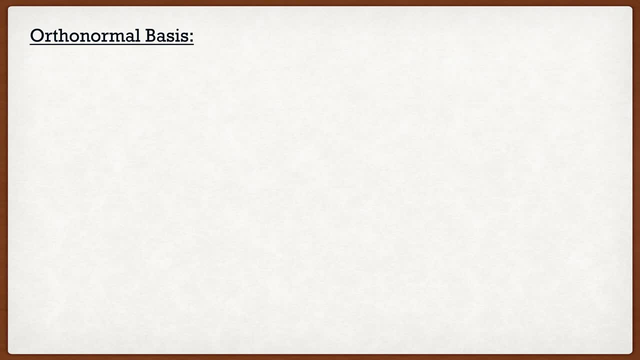 and again, this is going to be one of the more important concepts that we're going to use in both solid mechanics as well as finite element analysis. So an orthonormal basis set is a basis set B with basis vectors E1, E2, and E3, whose vectors are A, have a unit norm. So this is going. 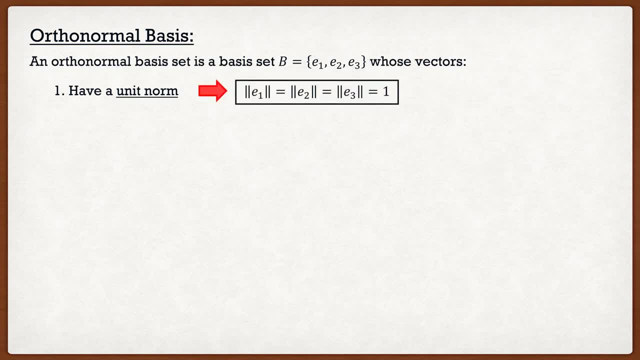 to be one of the most important ones. This basically means that the norm of E1, the norm of E2, and the norm of E3 are all equal to one. The second property is that they are all orthogonal to the norm of E3. So the angle between all three of these basis vectors is going to be 90 degrees. 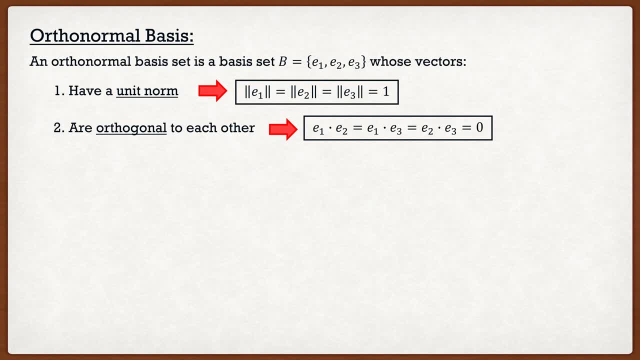 Therefore, we can say that E1.E2 is equal to E1.E3,, which is equal to E2.E3,, which is all going to be equal to zero. The proof for that was presented a few slides back Now. an example of this would be: 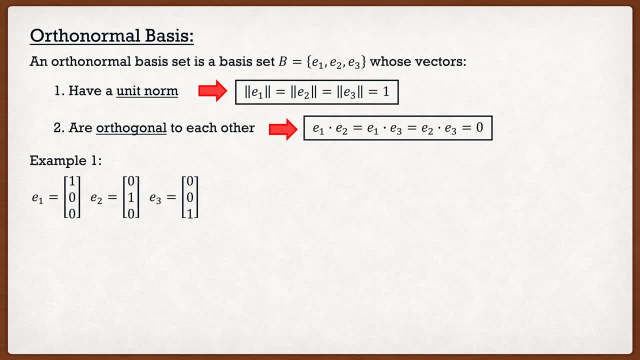 E1 is equal to 1, 0, 0,, E2 is 0, 1, 0, and E3 is 0, 0, 1.. If I were to draw a picture of this, well, it actually looks very familiar. This is the coordinate system you. 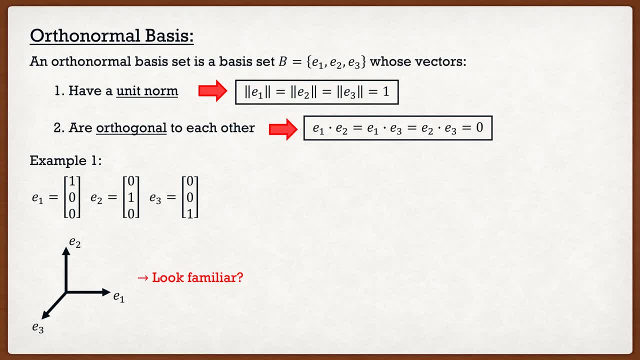 guys are probably most familiar with, because it's the standard 3D Cartesian vector coordinate system: Very, very simple but very, very powerful, because it allows us to express a lot of the mathematics as nice simple vector spaces. Now, we're not always restricted to this and, as you, 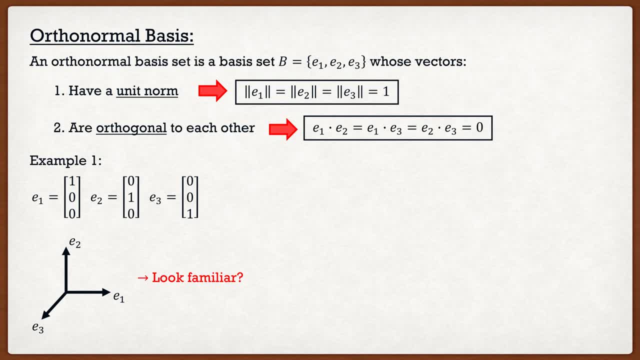 guys will see, in some examples we may need to pick a different basis set. So a different example of this would be: E1 is equal to 1 over square root of 2, 1 over square root of 2 and 0, while E2 is: 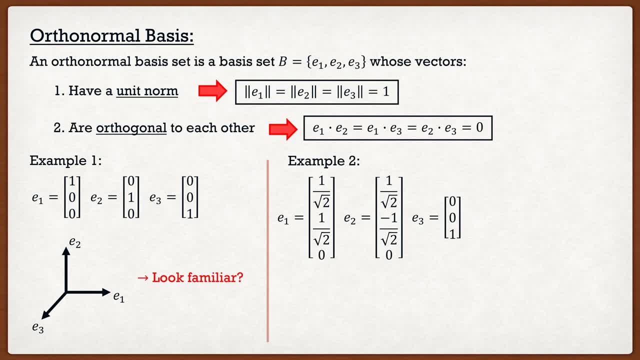 negative 1 over the square root of 2 and 0, while E3 is equal to 0, 0, 1.. This would look something like this and again, not all the time we need to use this, but there are some applications. 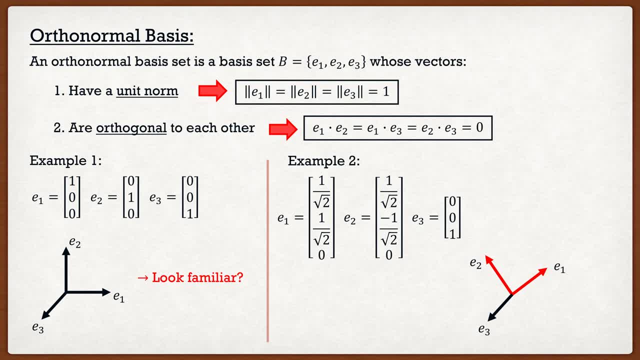 specifically, when a material has material properties that are different in different directions, It may be useful to pick a different orthonormal basis set than the one that we typically use. All right, so we're going to discuss more about this later, once we get into 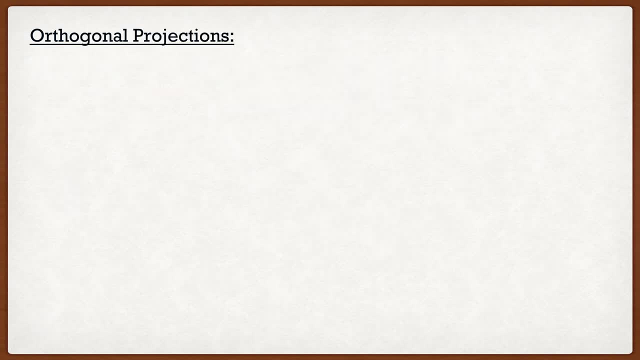 solid mechanics. The next thing we're going to discuss is orthonormal projections. So orthonormal projections of a vector u onto v can be used to determine the components of a vector u in the direction of a vector v. Now, I don't like it when people try and write mathematical. 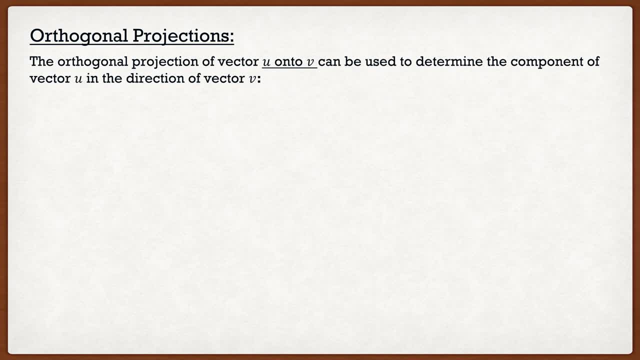 statements in words. like I did above, I always find it better to look at an example. So let's say that we have the vector u with components u1 and u2.. If I were to ask you guys what is the component of vector u in the direction e1, well, it's simple. It's just going to be equal to the. 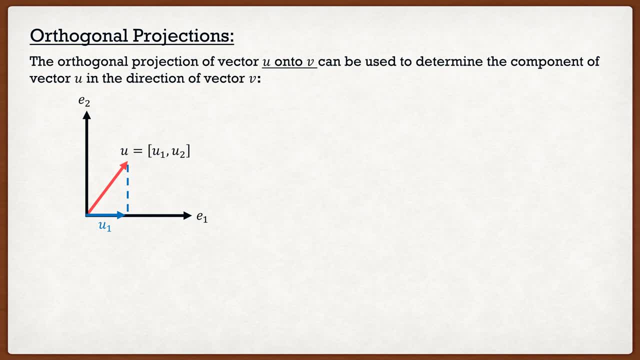 component u1.. Now if I were to ask you guys what is the component of vector u in the direction e1, again, very simple, We know it's just going to be the component u2.. But let's say I try and get. 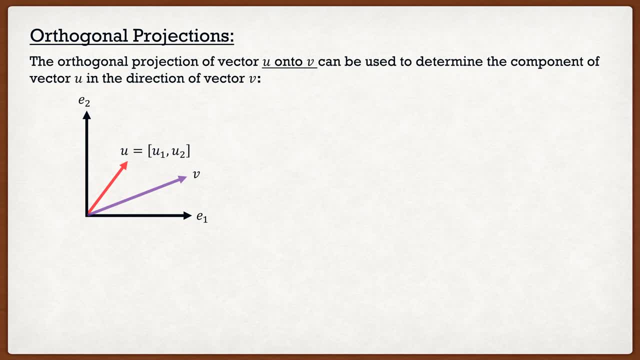 tricky and introduce a vector v, And then I would ask you guys, what is the component of u onto vector v? Well, that's what we're talking about when we discuss orthogonal projections. All right, so we're trying to find that component of vector u in the direction of vector v. Luckily for us. 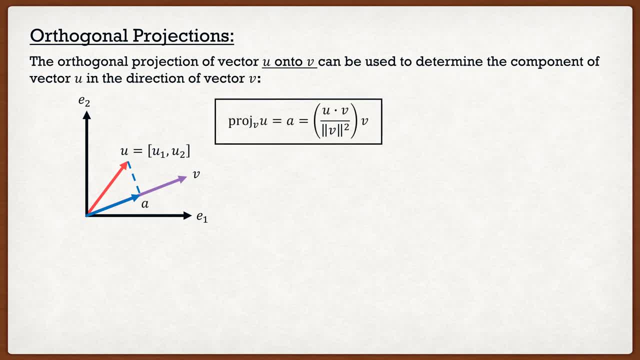 there is a nice formula for it. the projection of v onto u, which is the same as the orthogonal projection of vector u onto v, is actually equal to what I call vector a here, which is going to be u dot v divided by the. 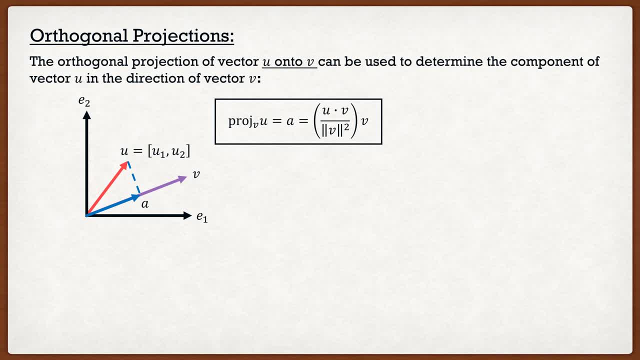 magnitude or the norm of v squared, then multiplied by the vector v. The key takeaway here is this: vector a is parallel to vector v. Now I can take it a step further and say: well, if I have a vector a that is parallel to v, I can also create a second vector which is going to be parallel. 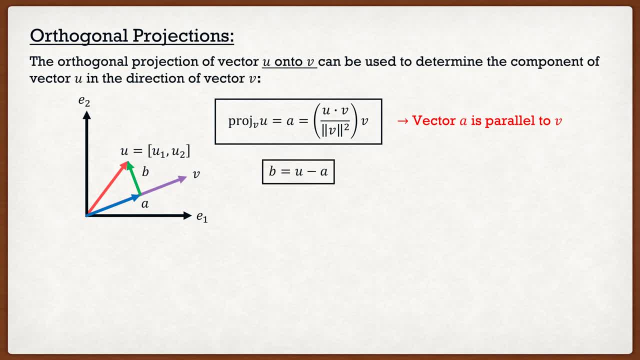 to v. So that'd be the green vector here, And let's call this vector b. Now, if I were to look at vector a, b and u as a whole, they form a nice triangle. Therefore they apply the laws of vector. 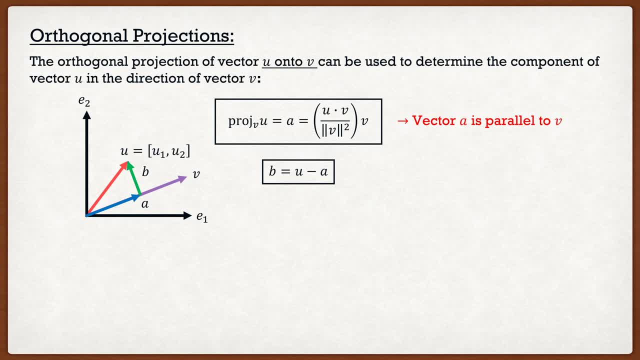 addition. Therefore, I can easily solve for vector b, as it's simply u, the vector u minus the vector a, And again the takeaway here is: vector b in this case is actually perpendicular to vector v. So a nice easy way to do this is: let's look at an example. So let's go with the orthogonal. 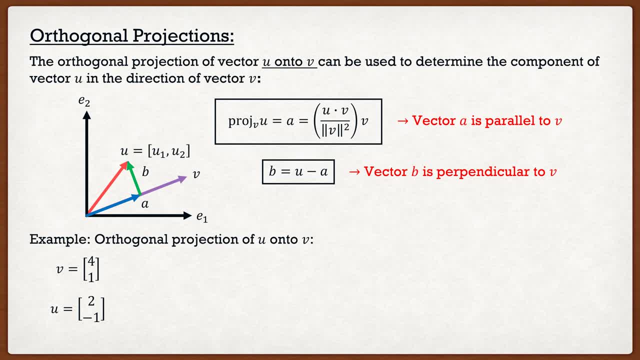 projection of vector a. So let's go with the orthogonal projection of vector b. So let's go with the orthogonal projection of vector u onto vector v. We're going to use the same vector components that we were using earlier. So if I wanted to find the orthogonal projection of u onto v? 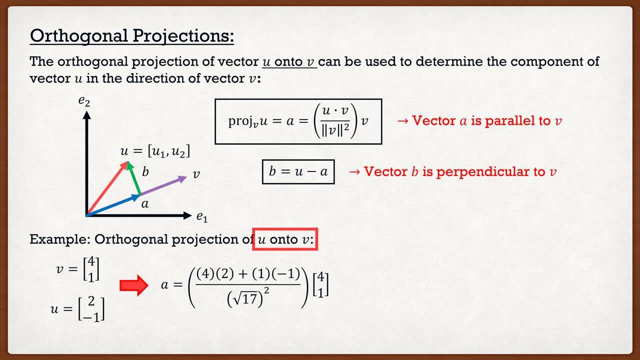 well, that's going to be that vector a that we discussed there. So what I'm going to do is I'm going to take the dot product of u and v, so 4 times 2 plus 1 times negative 1, and divide that. 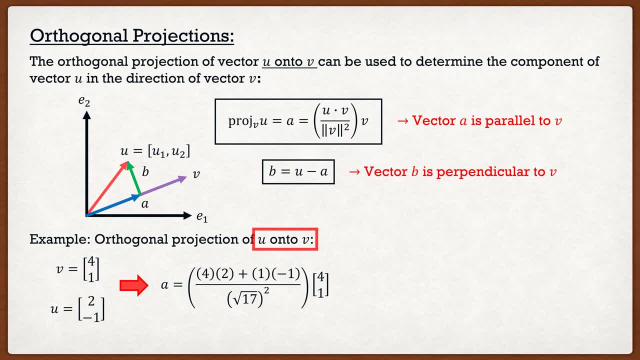 by the norm of v squared. So the norm of v is the square root of 17.. I'm going to square it And then finally I multiply it by the vector v. Now I put in a box there u onto v, because projections actually matter. which one are the? 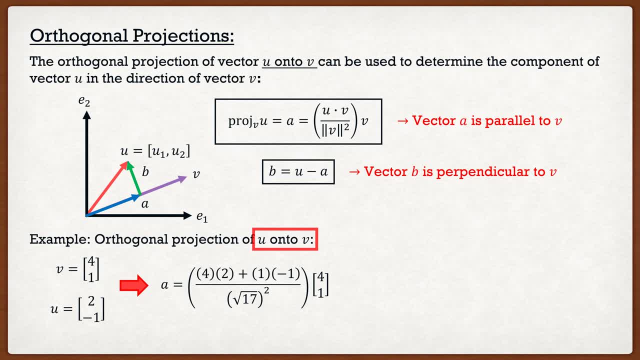 order of things, If I were to ask you guys the projection of v onto u, there would be different numbers in this equation, which makes sense, because if we look at the formula above, we can see that things are more dependent on vector v than they are on vector u. 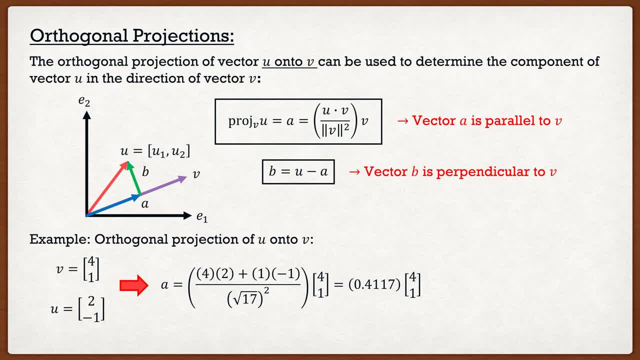 All right. so I can take this a step further. I can say: well, all that stuff in the nice brackets there, that's simply a scalar. So I end up with 0.4117.. I multiply that by a vector and I end up with a being a vector of 1.6471 and 0.4117.. 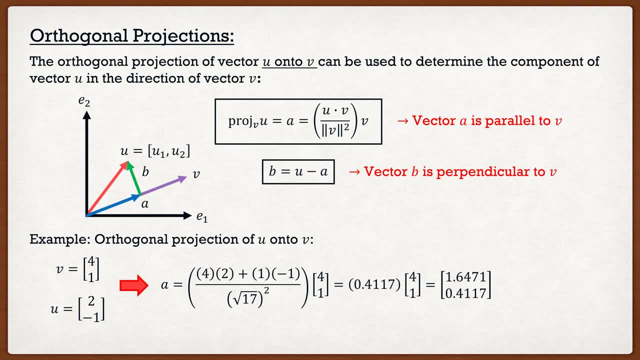 Again. another takeaway here is: when we do this orthogonal projection, we end up with a vector, All right. even though it looks like there's a lot of scalar components- which there is- we still end up with a vector, All right. so moving on, we now discuss something called the 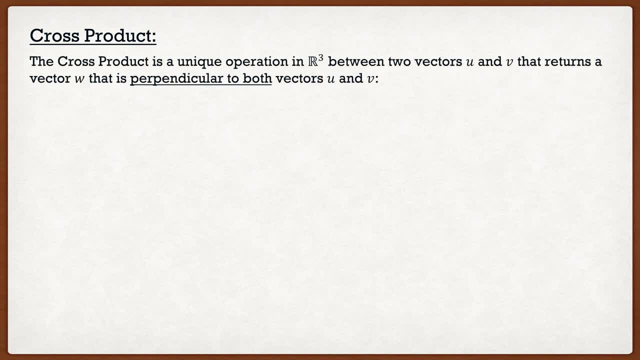 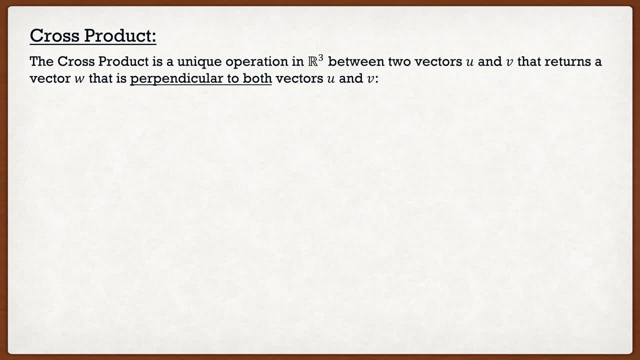 It returns a third vector, w- And here's the key- that is perpendicular to both vectors u and v. What exactly does this mean? Let's say that I have two vectors, u and v, and I were to cross them together. My resultant is a vector w, which is going to be perpendicular to both u and v. All. 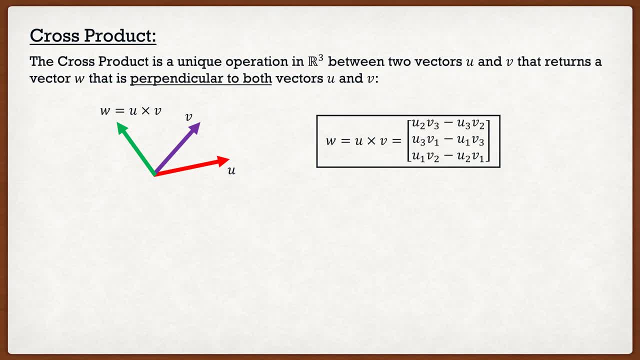 right. so there's the key here. it's perpendicular to both. Now the formulation for this. well, it varies. One thing I've learned as an instructor: there is a million different ways to calculate this stupid cross product. So I'm going to show you how to do it. So I'm going to show you how to. 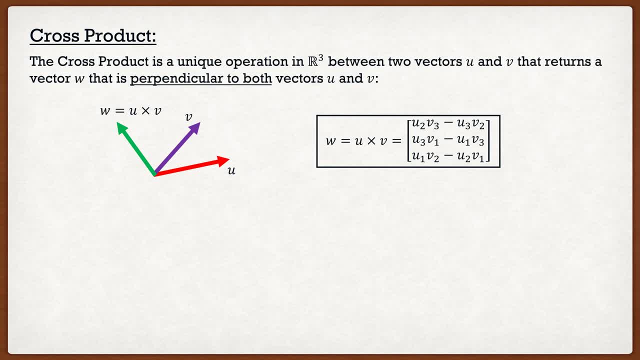 calculate this stupid cross product In component form. it's nice and simple. I can just say that w is going to be a vector of u2 multiplied by v3, minus u3 multiplied by v2,, etc. etc. But by this point you guys should have your own personal method of calculating the cross product. So I'm 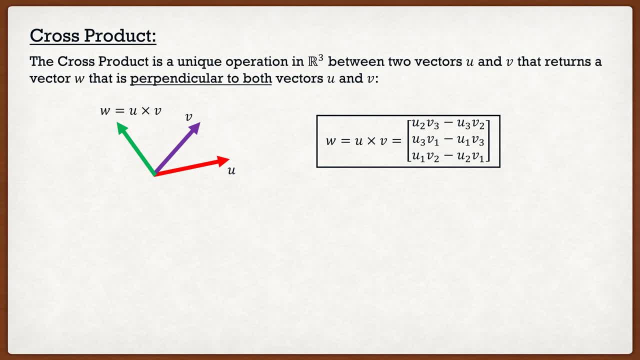 not going to worry too much there. Now, if we look at w, which is u cross v, it returns us with a vector. So if you guys take the cross product and get a scalar again, you guys probably did something wrong. So something to watch out for. 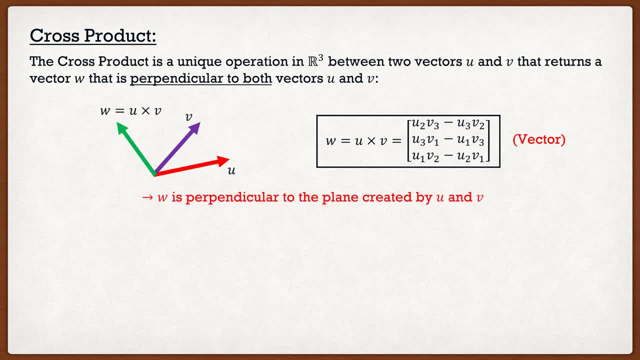 Now a couple properties. The first one is w is perpendicular to the plane created by u and v. that's going to be kind of the essential property that we're going to use. But there is a second property, which is, which comes in very handy when we start talking about solid mechanics proofs. 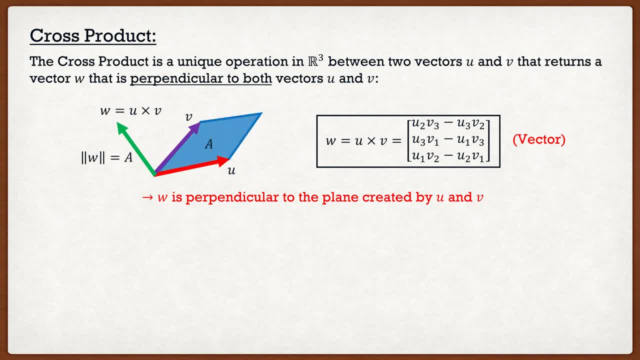 And that is this, the area of the parallelogram created by vector u and v, which is that blue parallelogram. there that's actually going to be equal to the norm of that cross product resultant vector w. So the norm of w in this case is actually going to be equal to the norm of the 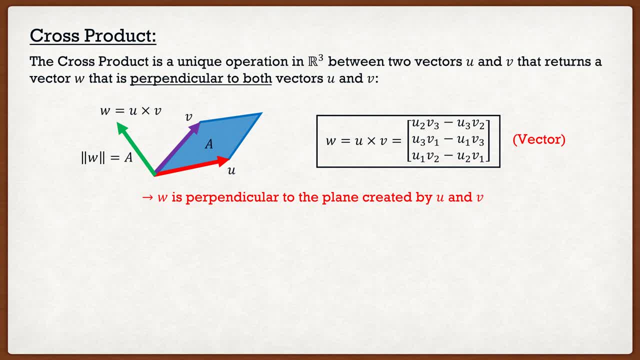 area of that parallelogram. This will come in handy once we start doing some more proofs in solid mechanics. Now, just like before, the cross product has a bunch of properties that we're going to discuss. The first one is the resultant vector. w is perpendicular to u and v. You guys are saying 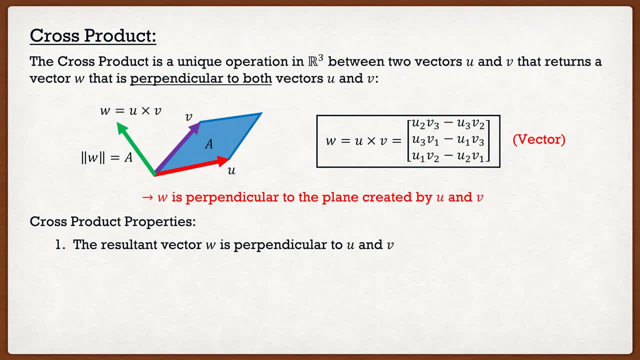 Clayton shut up. I've heard you say it a million times by now, But yes, it's very important, So please remember it And maybe I won't have to say it so much. All right, What exactly does this mean? 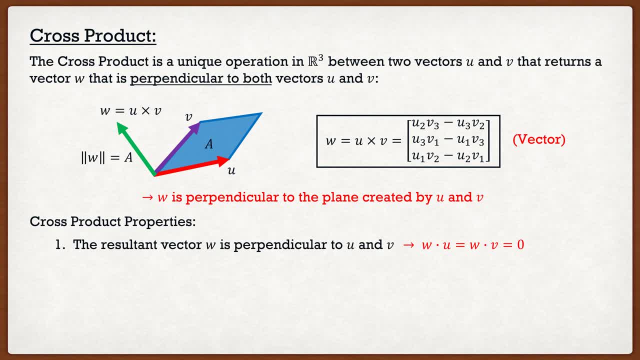 Well, it means that w dot u is equal to w dot v, which is going to be equal to zero. The operation here is skew symmetric, which means that u cross v is actually equal to negative v cross u. Again, something to be aware of, because a lot of people 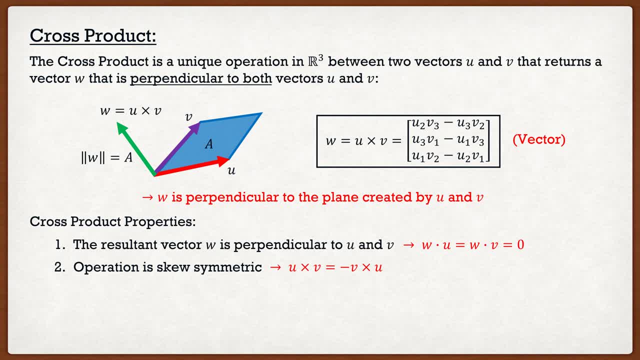 go u cross. v is actually equal to v cross u. they get it wrong. they get mad at me And I say, Oh no, no, I warned you about this, Remember, it is skew symmetric, So please keep that in mind. 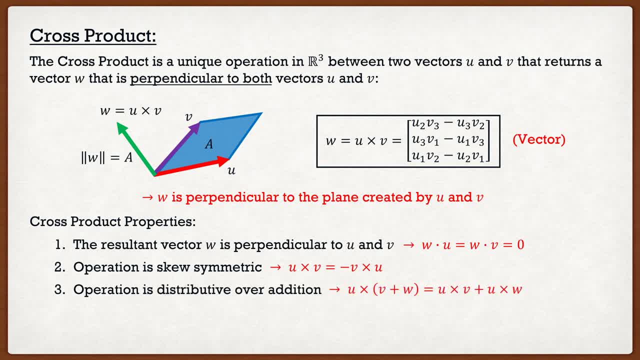 The operation is distributed over addition, which means that the following property holds: and the operation is compatible with scalar multiplication. Therefore, we can also utilize the following properties: And finally, there's a big, long sort of proof property. we're not going to get into that too much. it looks pretty gross, So we'll. 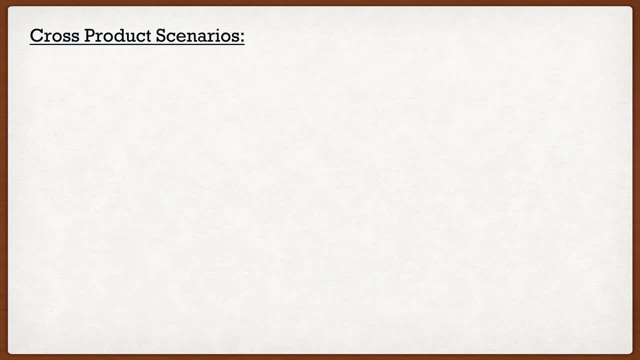 just, we'll just leave it as that, All right. So cross product scenarios: there's a couple scenarios that we're going to have to be aware of. The one is the cross product of basis vectors. If you guys were to look into tensor calculus or any of that crap, this comes up all the time. where that has. 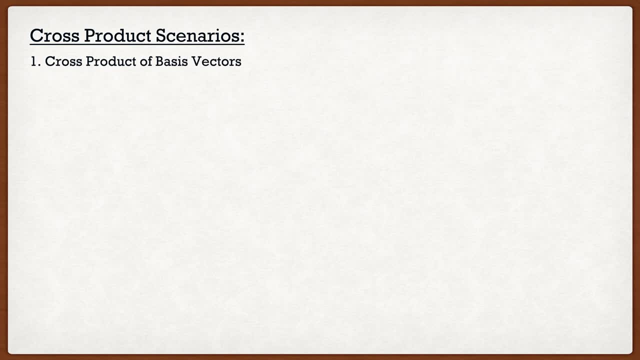 basis vectors crossed together, basis vectors dotted together. it's one of the fundamental and many of the proofs, But let's just take a look at what exactly it is. If I had the basis vectors e one and e two- and these are an ortho orthonormal basis set, well then, if I were to. 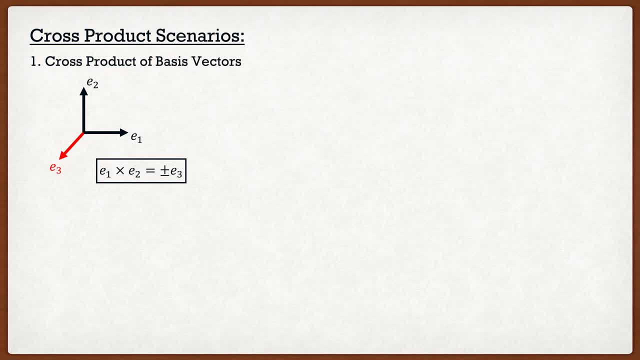 cross e one and e two together, I get e three as being perpendicular to both of them, which makes sense for an orthonormal basis set. I can do the same thing for basis set or basis vectors. e two and e three, I get e one. And finally, if I were to go e one and e three, well then, I get e two. 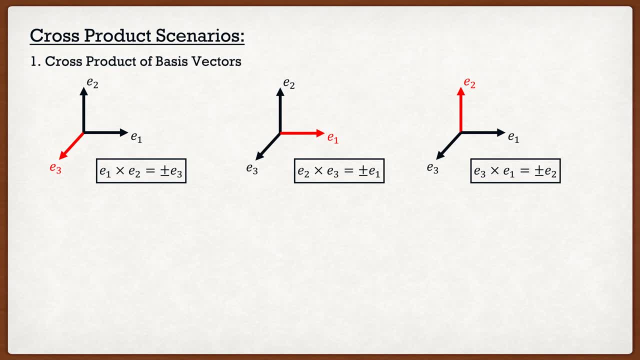 So that's something that's very easy to comprehend. The second lesser known property, of course, is going to be the cross product of linearly dependent vectors. So we already discussed what linearly dependent vectors are. they're vectors that can be written as linear combinations of one another. So if the vectors u 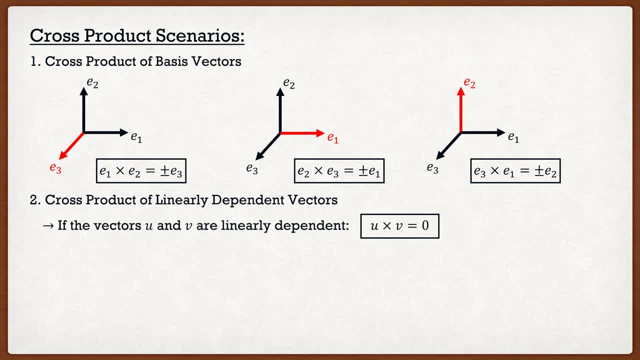 and v are linearly independent, or sorry, dependent, and make that very clear: dependent u cross v is actually going to be equal to zero. Very easy to see, because I'll just skip ahead, Because if I were to have the vector u and v which share the same direction, well, they don't. 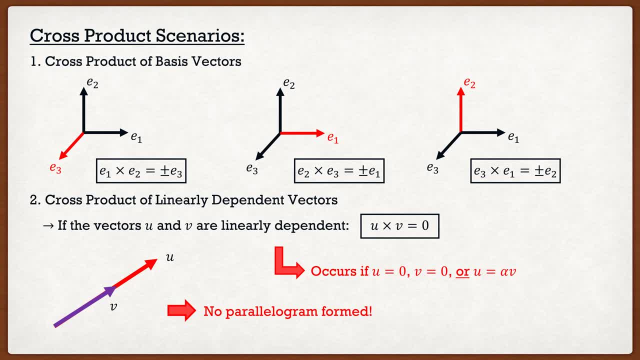 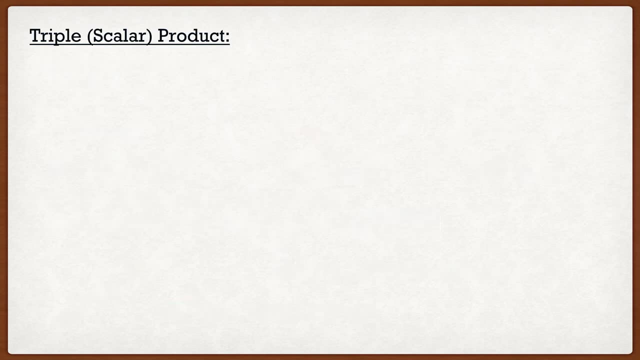 form a parallelogram. So therefore the area is going to be equal to zero, And this occurs if the vector u is equal to zero, the vector v is equal to zero, or u is equal to some scalar multiplied by v. So pretty easy to see. Next we're going to talk about the scalar, or the triple product, or 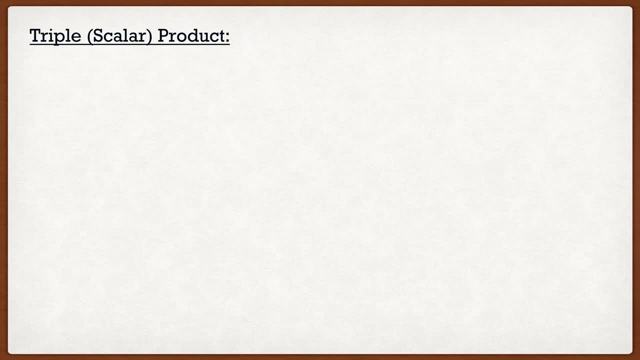 that triple scalar product. I've seen the definition vary or the name of it vary between sources, And this is basically the volume of a parallel pipe created by the vectors u, v and w using the triple product or the triple scalar product, which is this nice ugly formula, right? 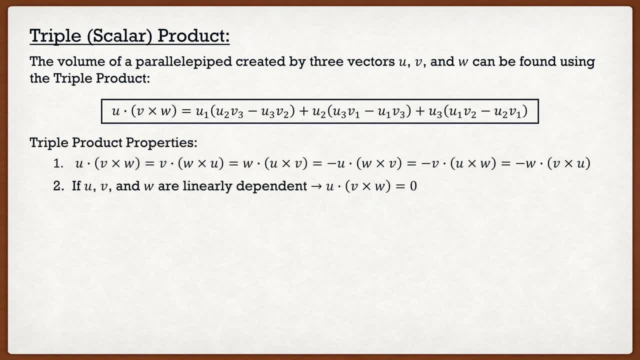 here, And of course, it has some properties which I'm not going to really get into. This plays a little bit of a role, as you guys will see later, when we're talking about linear maps, but it's not too, too important, So I'm just going to leave it be for now. Now, the last thing that we're going. 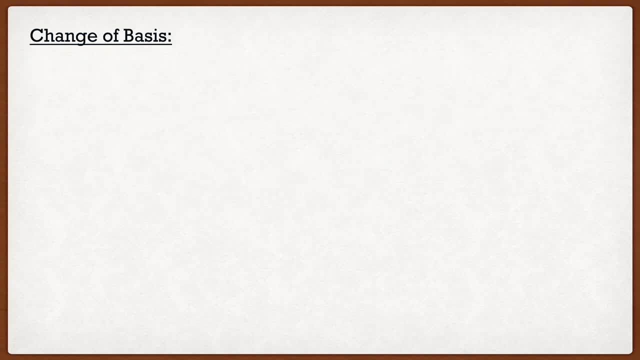 to discuss in this lecture, which is very important, is a change of basis. So this is going to be one of the more critical things, especially when we start talking about solid mechanics. So the basis of a vector depend on the selected basis vectors, And this makes sense In some scenarios. 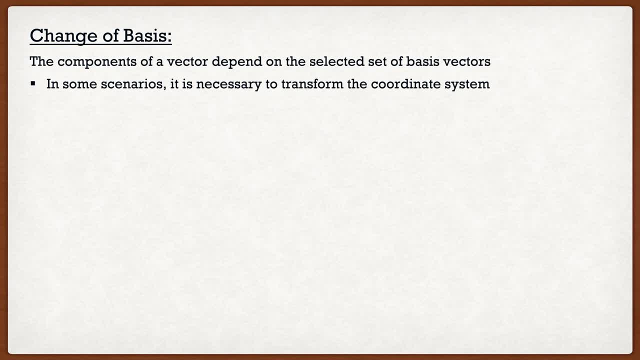 actually it might be necessary to transform our coordinate system. Now this is when you guys say: Clayton, hold up, slow down. What do you mean? transform the coordinate system? Well, let's say I had the basis vectors e1 and e2.. And in that basis set I had a vector u which is equal to. 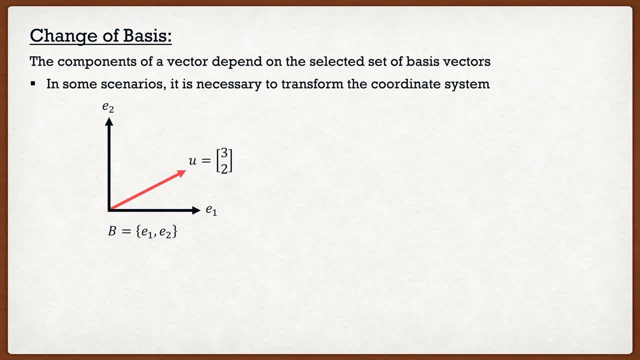 three comma two, what a change of basis is, or a transformation of the coordinate system. As I take this basis set, I transform it by what we call a coordinate system And what we call a coordinate transformation, matrix q. And then I end up with the following where, as I can see here, I took my 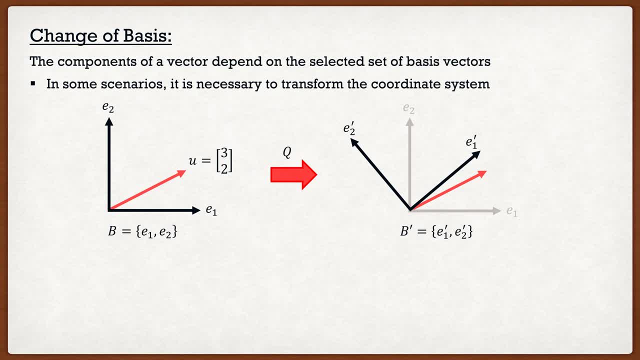 two basis vectors, e1 and e2, and I rotated them counterclockwise. Now, the rotation doesn't always have to be counterclockwise. I could have rotated it clockwise if I wanted to. this is just for the purpose of illustration. Now, if I look over here, I say Alright, I can see that e1 and e2 have now. 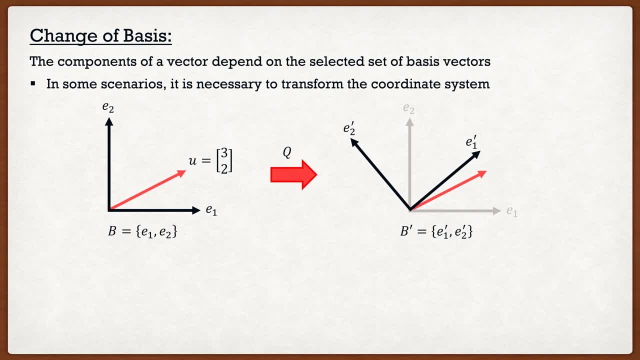 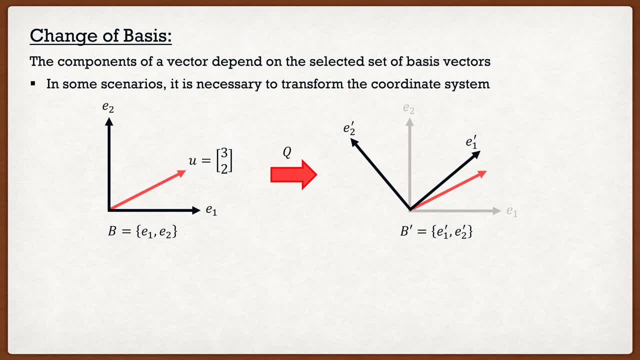 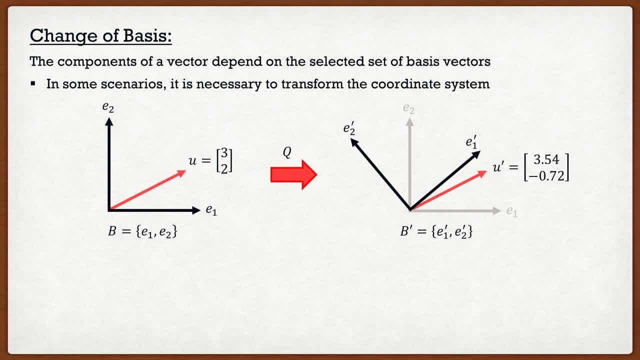 0.72.. So here's the key here: that the vector didn't change direction or the vector didn't move. However, since we changed the basis vectors, we actually changed the components of that vector, And if we wanted a relationship between u and u prime, it's actually going to be. 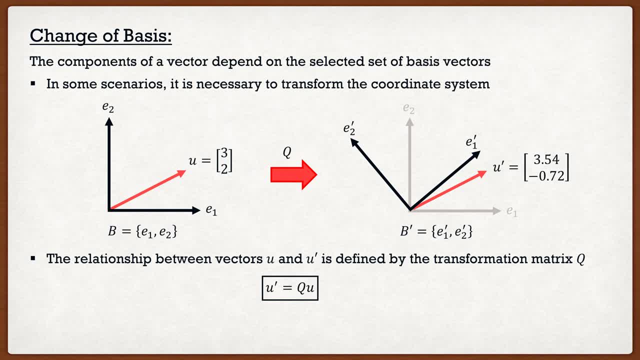 very simple. It's defined by the coordinate transformation matrix q, where u prime, which is the vector in the transformed basis set, is equal to q multiplied by the vector u, which is the vector in the original basis set. So we look at this and we say, Alright well. 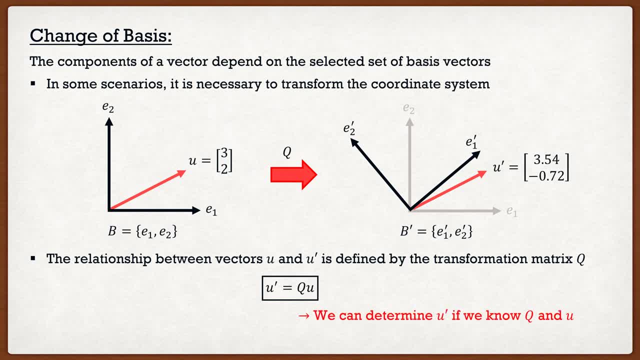 if I wanted u prime. it's actually not too bad, because all we need to know is both q and u. Now, when we see problems, we're always given u. that's our original vector. that's not going to be a problem. What we don't really know is: what is q? What is that q? What is that q? What is q? 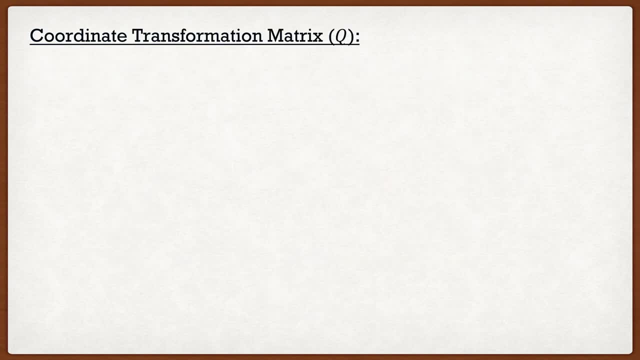 What is that coordinate transformation matrix? So let's discuss the coordinate transformation matrix q In general and the general sense. the coordinate transformation matrix q can be calculated from the two basis sets. So we have our basis set, which is the original basis set. 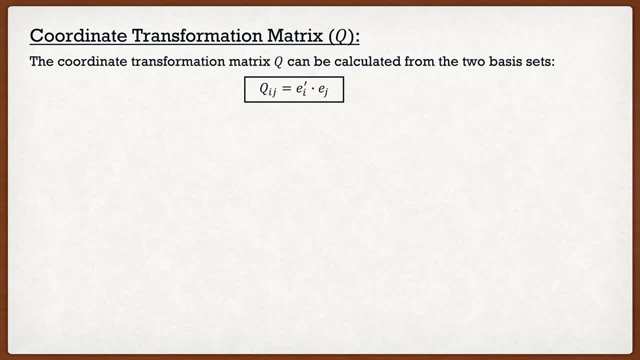 e1 and e2.. And we have a second basis set which I call e1 prime and e2 prime And the components of the coordinate transformation matrix q, which is qij, can simply be found by dotting ei prime j. Now when I look at this formula- let's be honest- it looks really gross. It's very hard to. 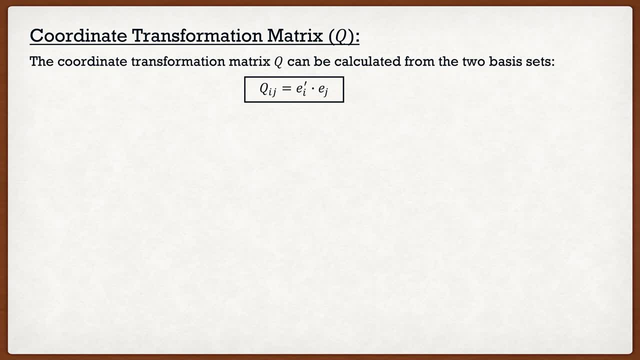 just look at this form, the picture, what exactly it's doing. So what we're going to do is a nice example of a 2d counterclockwise rotation. So let's say that we had our original basis vectors e1,, which is one, zero, and e2,, which is zero, comma one, And we transform this into the new 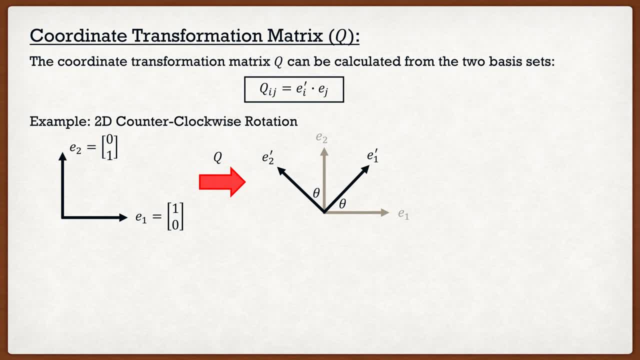 basis set e1 prime and e2 prime, So of course we're rotating this counterclockwise by a magnitude of theta. So the first thing that we're going to want to know is: what are the components of e1 prime and e2 prime? Well, they're actually very simple. If I were to create a nice right triangle with 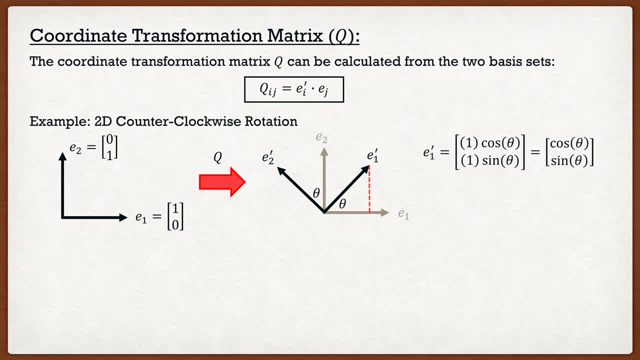 e1 prime and the original basis vector e1,. well, I can see that the horizontal components of e1 prime is simply going to be one multiplied by cosine of theta. The reason why it's one is because the hypotenuse of e1 prime must be equal to one, because, again, if it's an orthonormal basis, 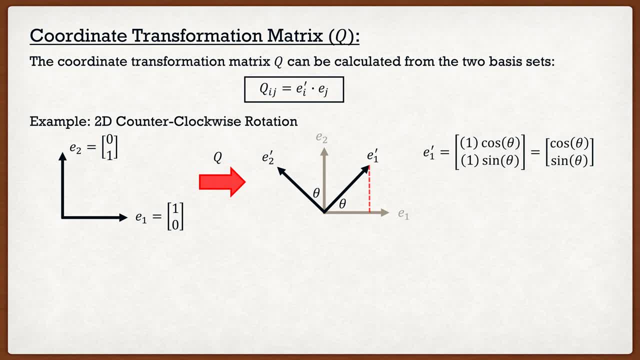 vector, it must be equal to one. So it's going to be one multiplied by cosine of theta, which is just going to be cosine of theta. If I wanted the vertical components of e1 prime, it's again just going to be one, which is the hypotenuse, multiplied this time by sine of theta. So I just get sine of. 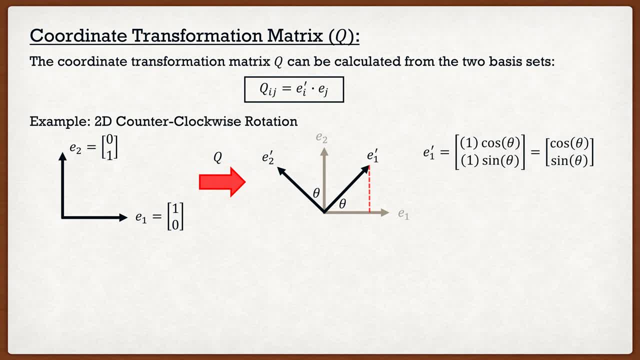 theta. So e1 prime cosine theta, sine of theta. not too difficult. We can do the same thing over here for e2, where we go, e2 prime is going to be equal to negative one, And the reason why it's. 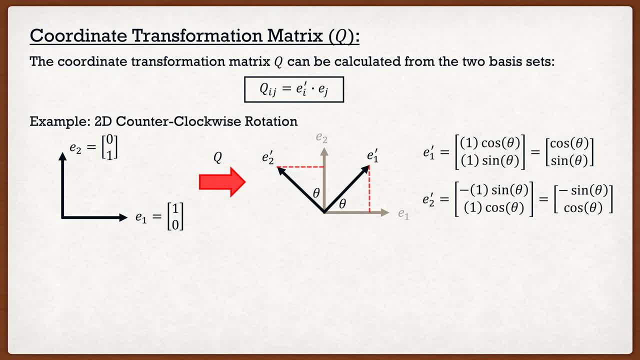 negative one is because now e2 is going in the opposite direction of the original basis vector. So e1 prime is going to be the original e1 multiplied by sine of theta, which gives us negative sine theta, And then the vertical components just going to be equal to cosine of. 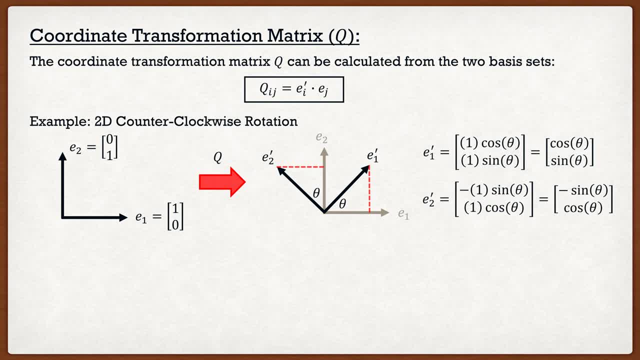 theta. Now that we found what those components are, we can actually find our coordinate transformation matrix q. So, for instance, if I want a q11, that's going to be e1 prime dotted with e1. So it's going to be cosine of theta times one plus sine of theta times zero, which. 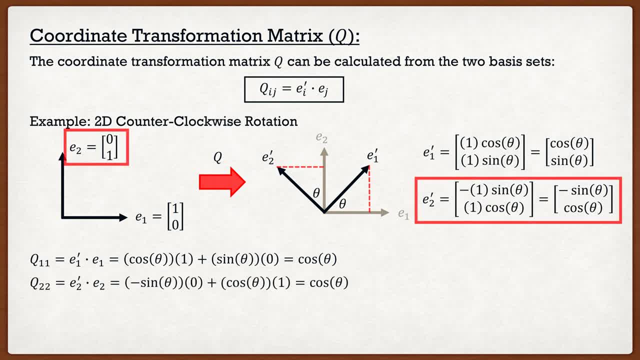 leaves me simply with cosine of theta. On the other hand, if I want a q22, it's going to be e2 prime dotted with e2, which gives us negative sine theta times zero, which is going to be zero, plus cosine of theta multiplied by one, which is simply just going to 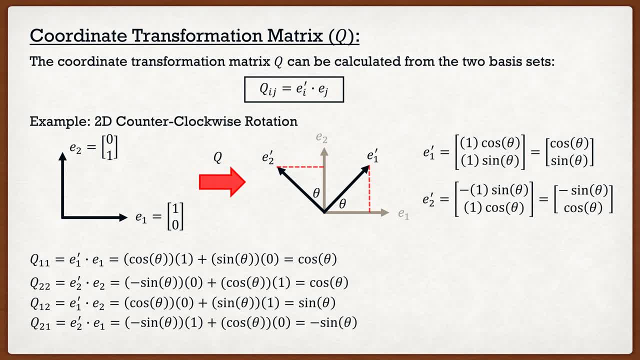 be cosine of theta. Now if I wanted q12 or q21, as I can see, all I have to do is put in the correct entries of the basis vectors: do the dot product. I'm left with sine theta and negative sine theta. 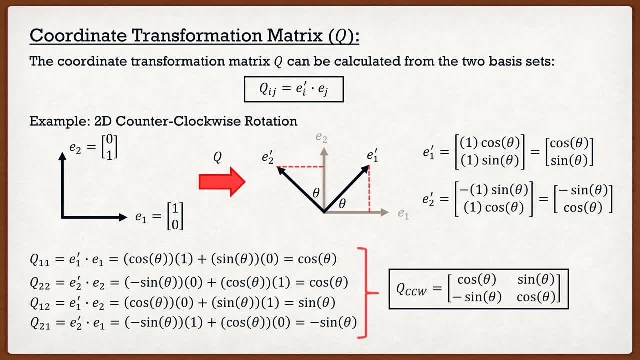 Therefore, my coordinate transformation matrix q for a counterclockwise rotation in two dimensions is just simply going to be cosine theta sine theta, negative sine theta and cosine of theta. Now, the one last thing that I want to try and touch upon before we end this lecture is 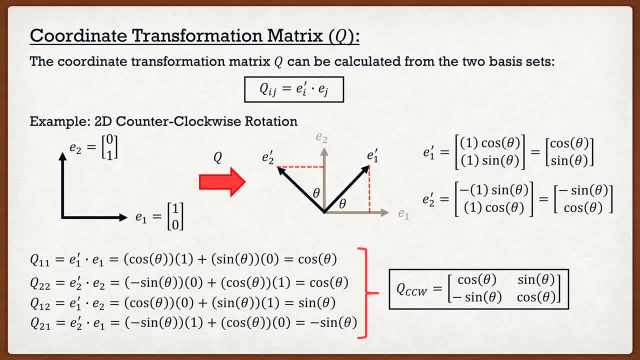 coordinate transformation matrix. Well, we haven't really discussed what a matrix is And, as you guys are going to see, a matrix is a type of linear map which is going to be the focus of our next lecture. So, if you guys want to stick around for more information about transformation matrices, 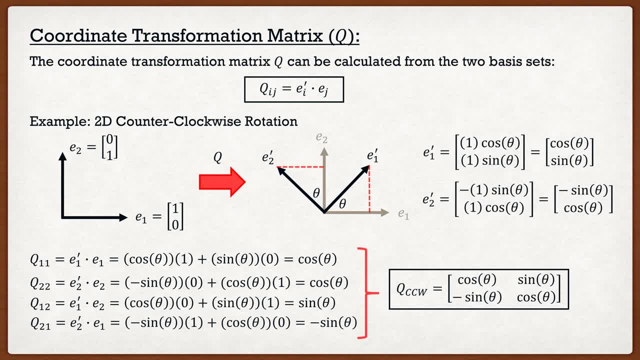 transformation matrices and stuff like that. that'll be in the next lecture, But that is it for this lecture. So I know it was pretty boring. Linear algebra in general I find pretty boring, So hopefully you guys made it through. Okay, Hopefully you're not sleeping. 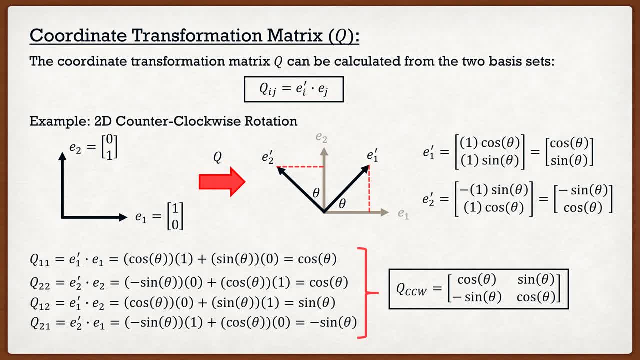 on me. Well, let's be honest, you guys probably are, But that's okay. Again, linear algebra: not super important for this course. it'll just help you guys make sense of the proofs that we do later on. So, thank you guys so much for listening. I really appreciate it. I will see you guys in the